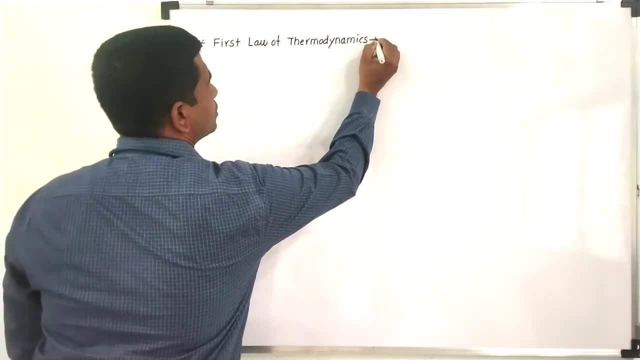 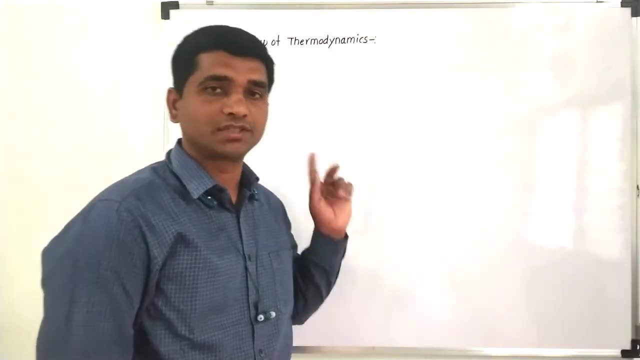 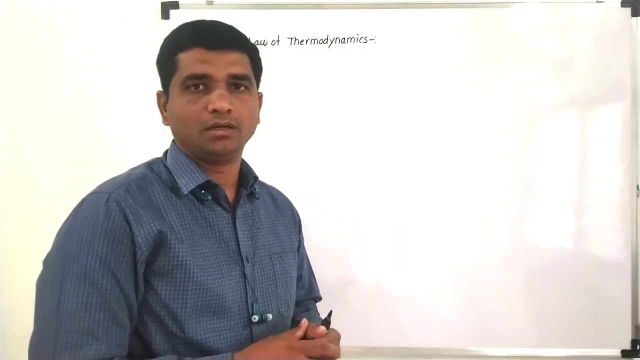 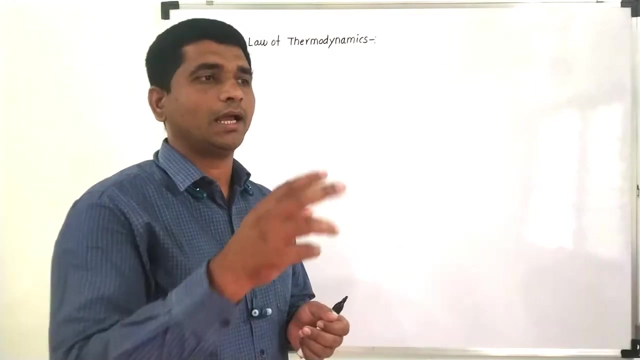 Actually this first law of thermodynamics. it was proposed before the zeroth law of thermodynamics. In our earlier session we have discussed what is zeroth law of thermodynamics and we have discussed the concept of thermal equilibrium. If two bodies are in contact, if first body is in thermal equilibrium with the third body, third body is in thermal equilibrium with the second body, and if A and B are not in thermal equilibrium or they are separated, isolated from each other. 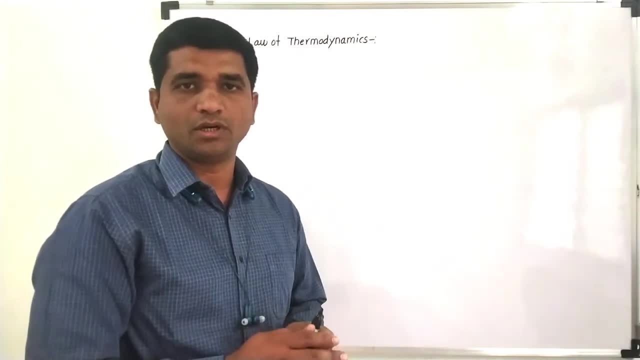 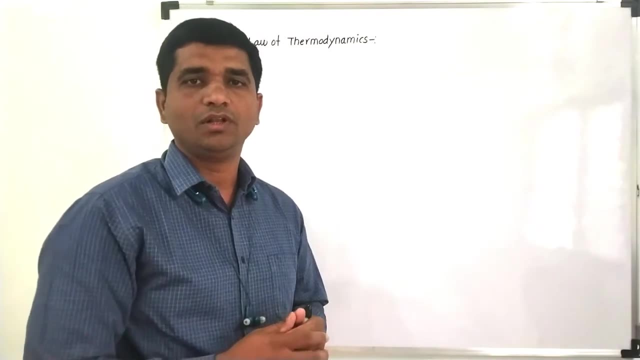 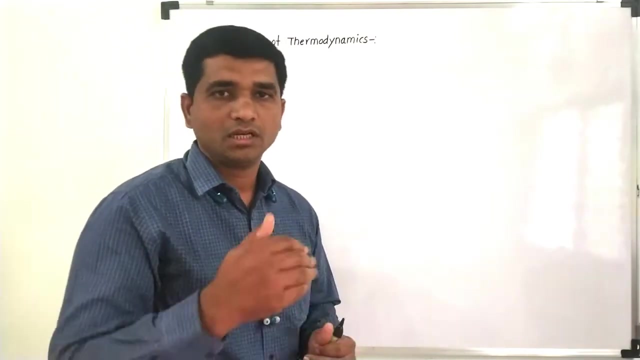 though they are not in thermal, they are isolated from each other. by using the equilibrium between first and second or second and third body, we will be having a thermal equilibrium between first and second body That we had seen in the zeroth law of thermodynamics. Now, in today's session, what we will be discussing that is the first law of thermodynamics. 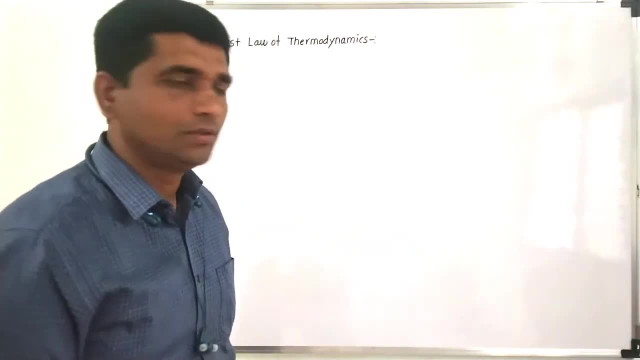 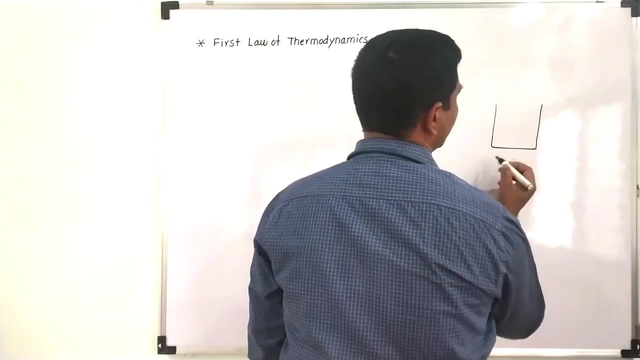 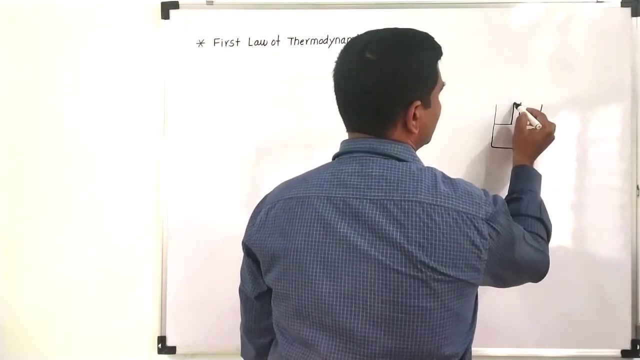 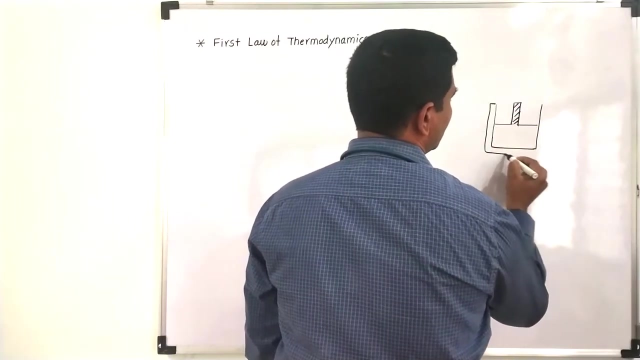 For to discuss the first law of thermodynamics, what we will do, what we will be considering and one system. for example, let us consider this container is there which is fitted with this piston. let us say this is a container which is fitted with this piston. so let us say this is a piston and this container, it is having gas enclosed in it. let us say this is the gas which is enclosed in this system. 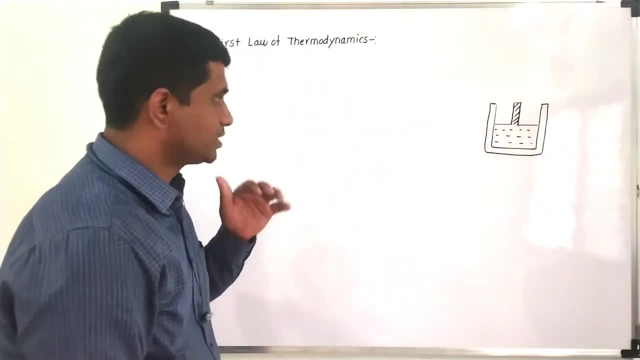 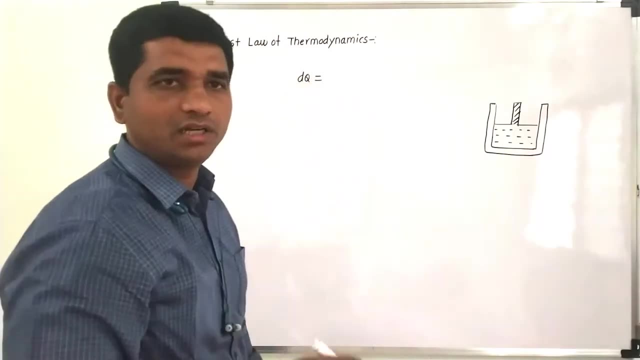 Now what first law of thermodynamics tells us? that suppose the amount of heat is given to the system, let us say dq is the amount of heat it is given to this system. so what will happen as we provide the heat to this gas? 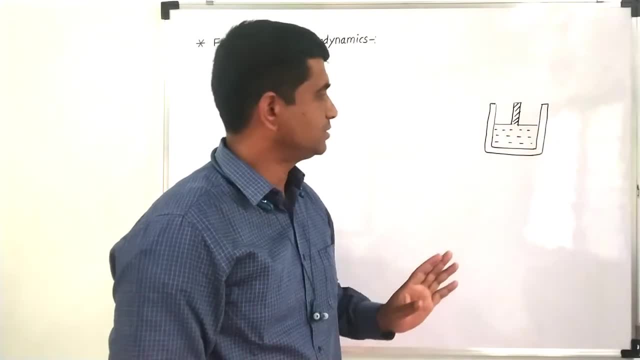 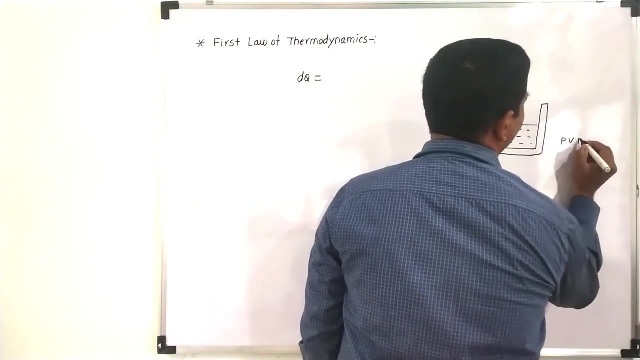 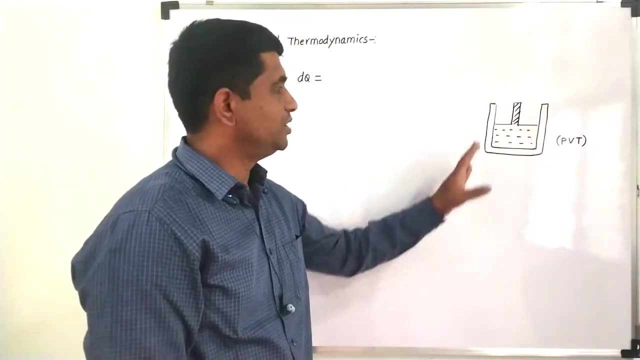 so let us consider: this container is having certain amount of gas, okay, which is having this. let us say initial volume and pressure. let us say it is having pressure T, volume B and temperature T is the parameters which are there for the specification of this state of the system. 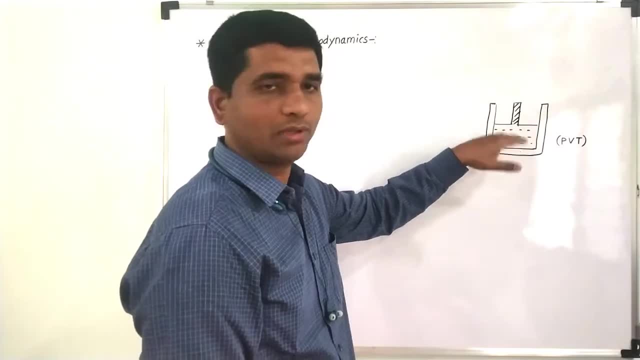 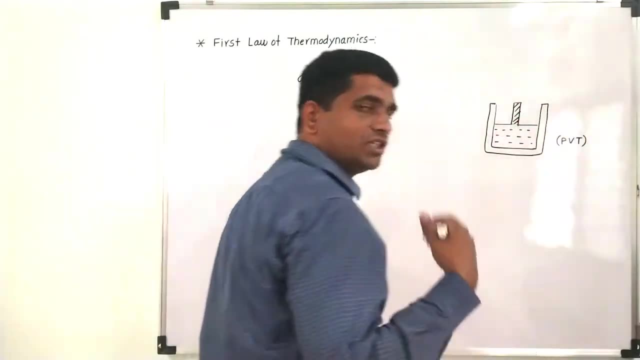 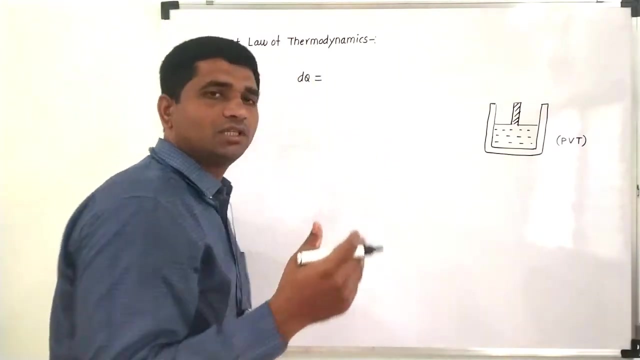 As we provide some internal heat to this system. as we provide the heat to this system, what happens is that its volume increases. its volume increases and its temperature also increases. okay, and that formulation. it was proposed in the form of first law of thermodynamics, which is nothing but the actually the extension of a first law of thermodynamics. 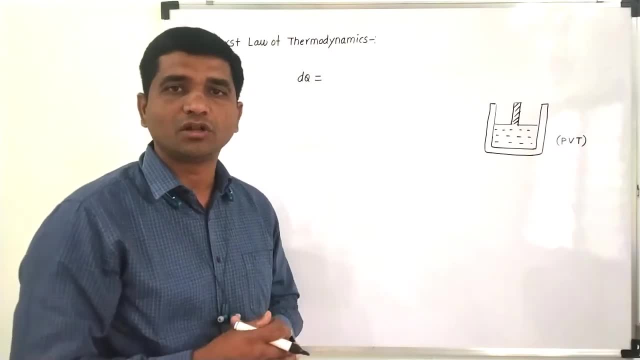 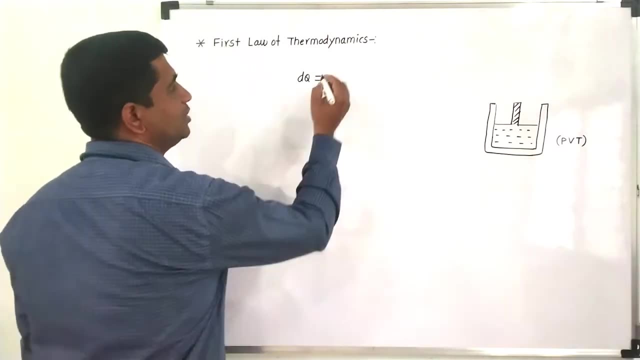 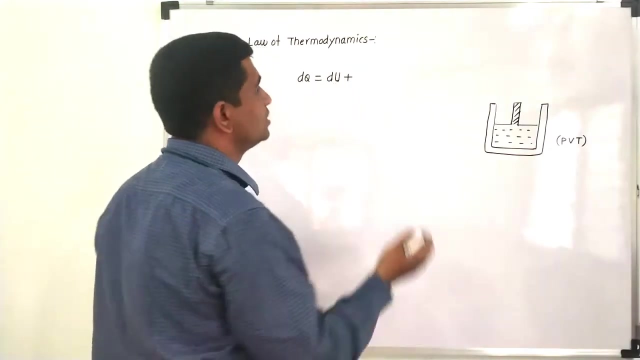 it is an extension of. it is an extension of law of conservation of energy. what it tells us? that the amount of heat given to the system, the amount of heat given to the system, it is used for two purposes. the first purpose is to increase its internal energy and to perform some work done. 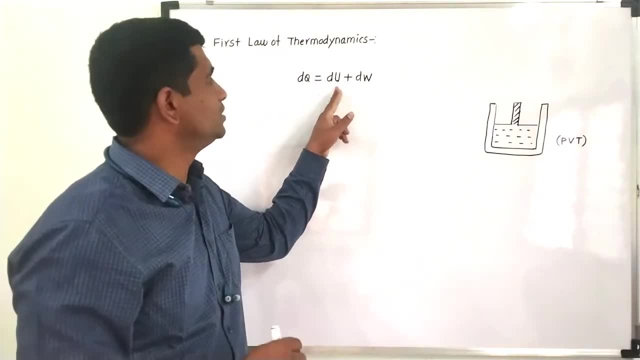 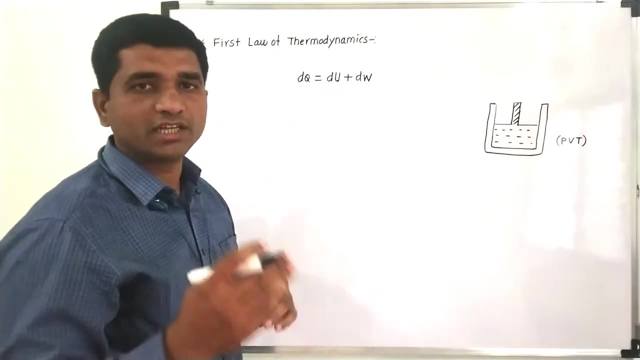 the amount of heat given to the system. it is used for two purposes. one is to increase its internal energy, to change its internal energy and to perform some external work done. okay, so that is the mathematical expression for the first law of thermodynamics. 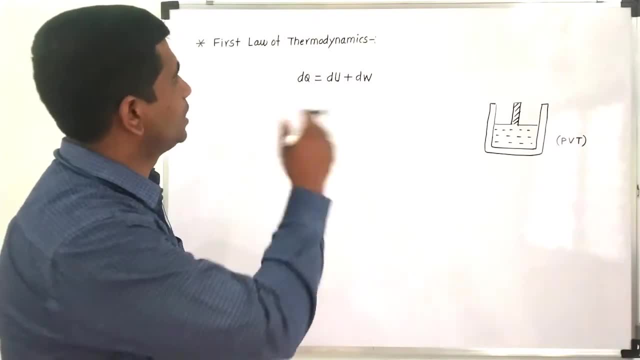 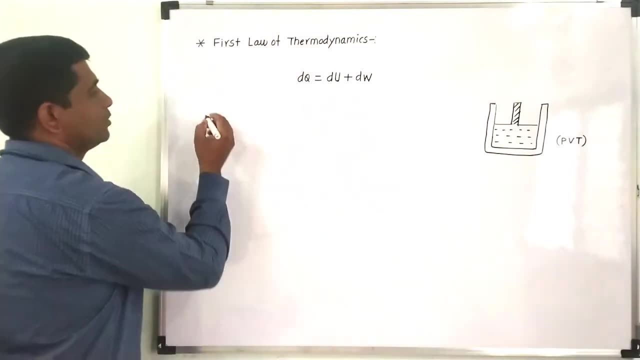 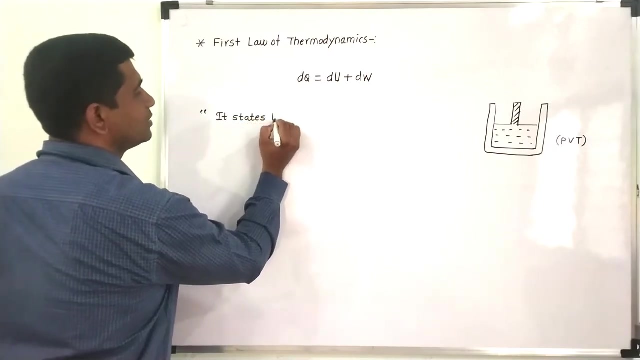 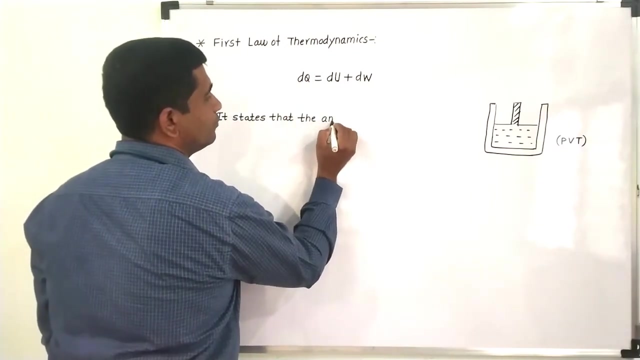 from this one we can. we can prepare mathematical, theoretical statement for the first law of thermodynamics. so first of all, we will note it down. what is first? what statement first law of thermodynamics tells us? okay, first law of thermodynamics, it states that. it states that it states that the amount of heat, the amount of heat, the amount of heat. 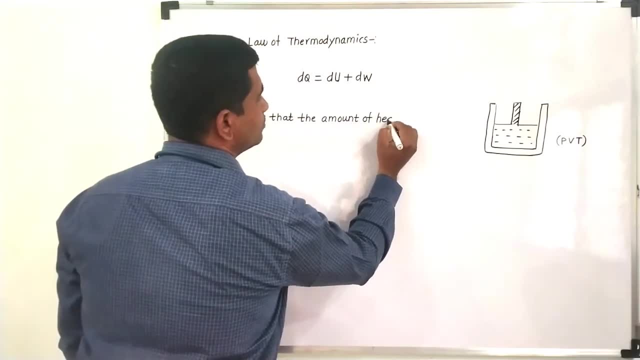 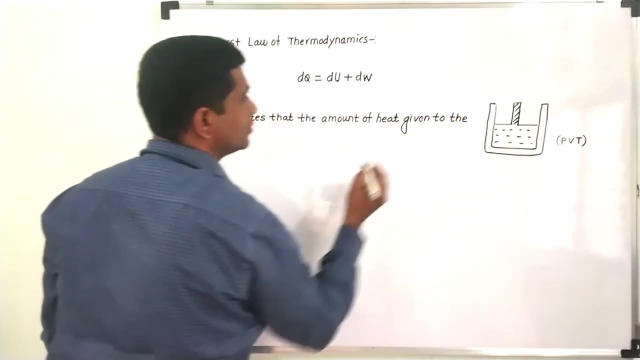 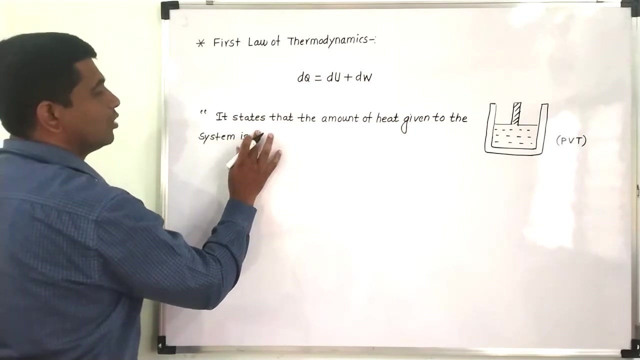 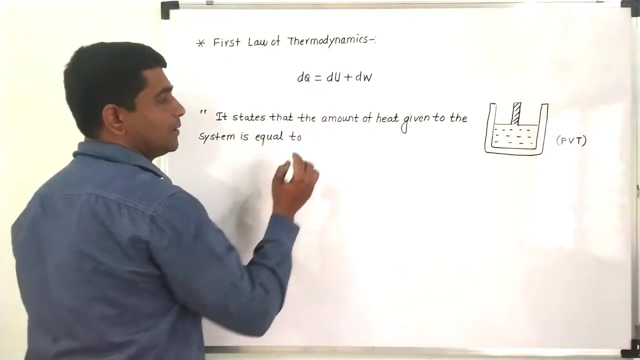 amount of heat given to the system. amount of heat given to the system, given to the system is used, or is equal to. is equal to. is equal to the algebraic sum of. is equal to the sum of. 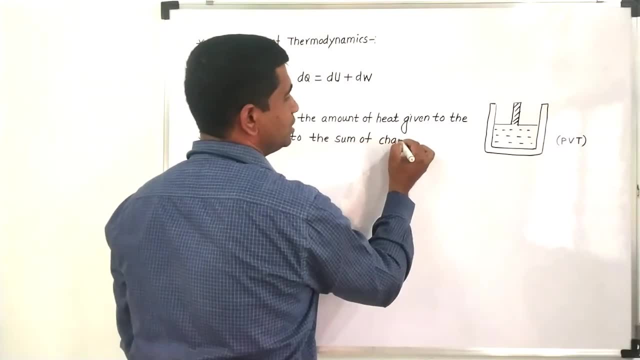 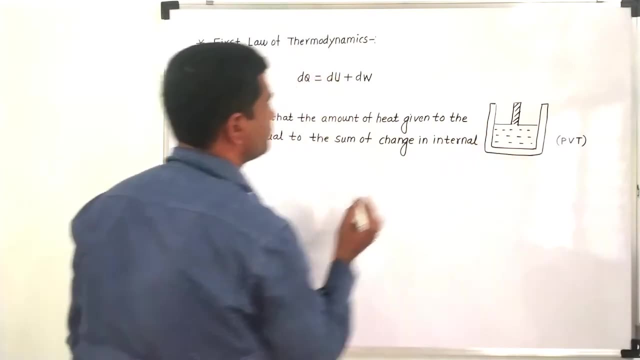 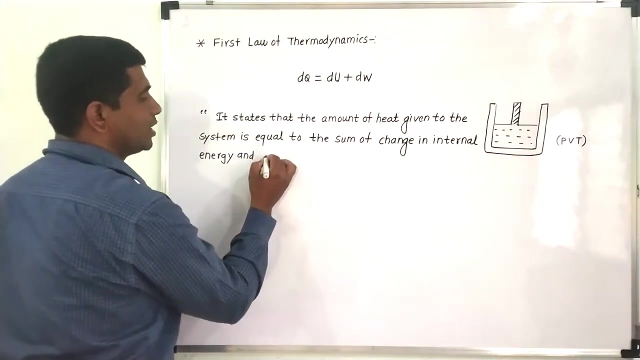 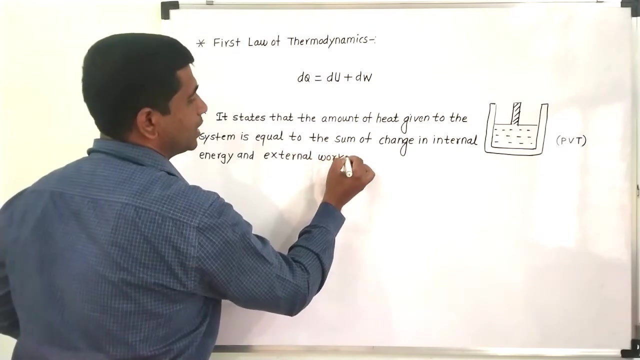 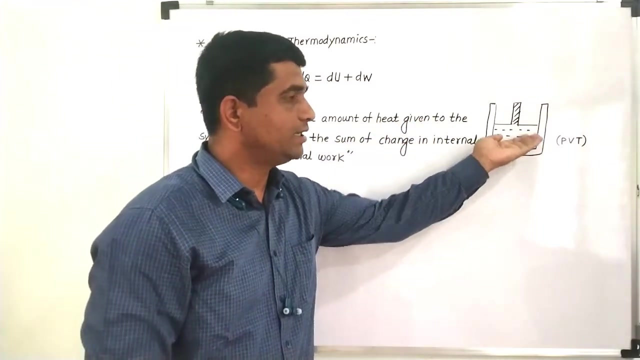 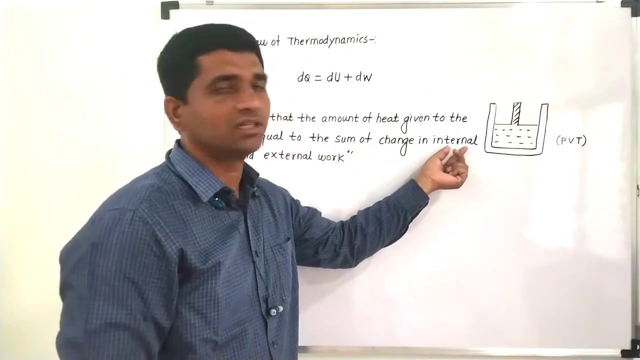 Change in internal energy, change in internal energy, change in internal energy and some external work done and external work done okay. So from this one we can see what happens to this container, See the amount of heat given to the system. so if I heat this gas which is inside this container, so what will happen? due to that one, its temperature will increase, and we know that temperature is a internal energy, is a function of temperature. 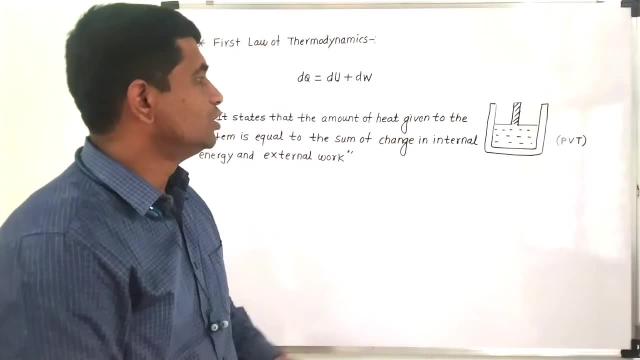 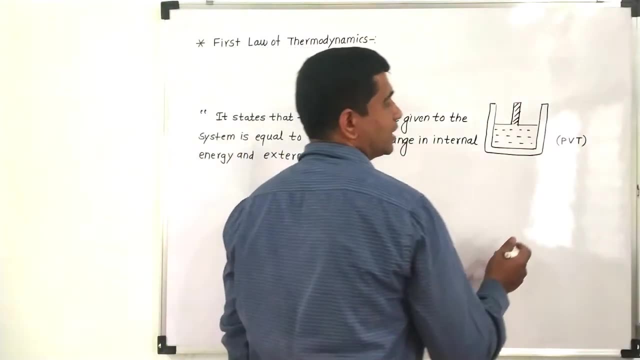 So as temperature increases, internal energy increases. okay, So its internal energy will increase, so DU will increase and external work done. How this external work can be calculated, See, suppose, the initial volume of this one. let us say P1,, V1,, T1.. 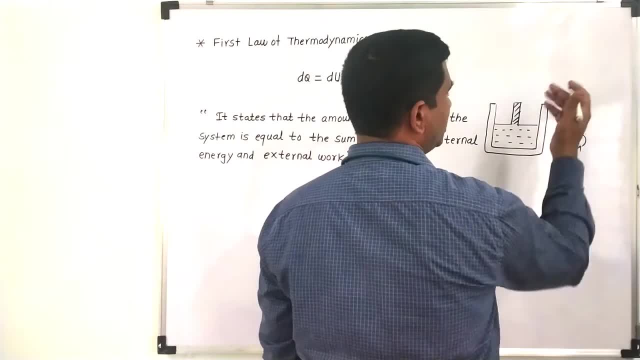 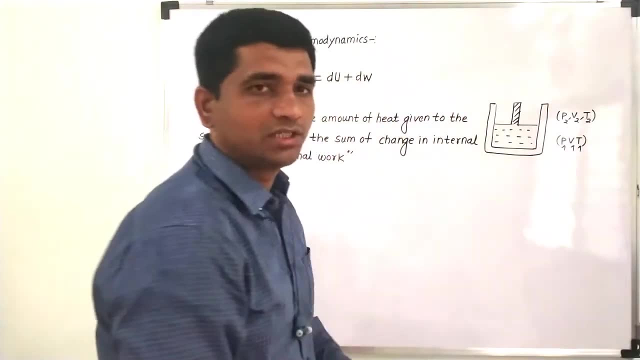 What is the pressure volume and temperature of this gas? So if I heat this one, let us say P2, V2, and T2 will be the pressure volume and temperature of this system after providing a certain amount of it. 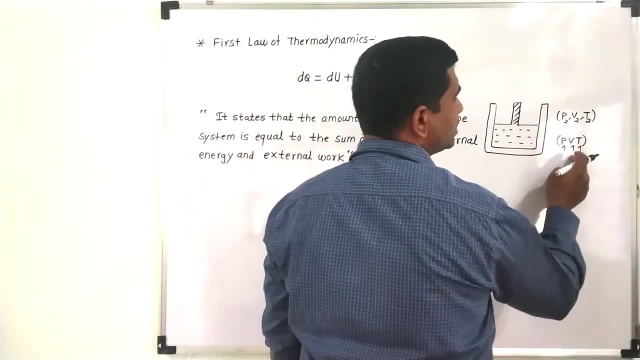 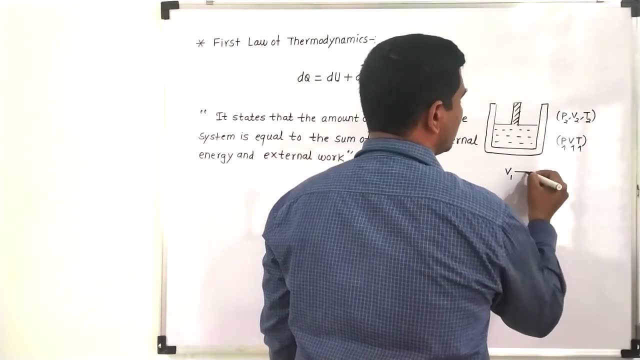 So if you consider over here, its volume is increasing from V1 to V2.. Its volume is increasing from V1 to V2.. So if I am saying that the gas is expanding, the gas is expanding, In that case you are changing volume. 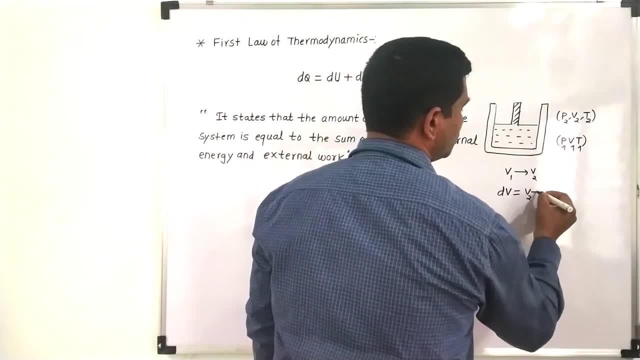 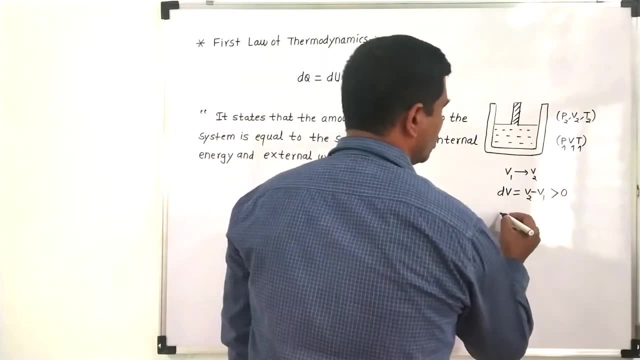 You are changing volume, It will be what V2 minus V1.. So if it is an expansion, then this quantity will be greater than zero. It will be a positive quantity And we know the work done. we know the work done which is a product of force into displacement. 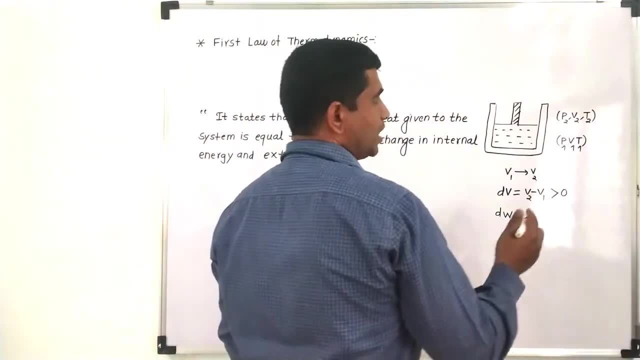 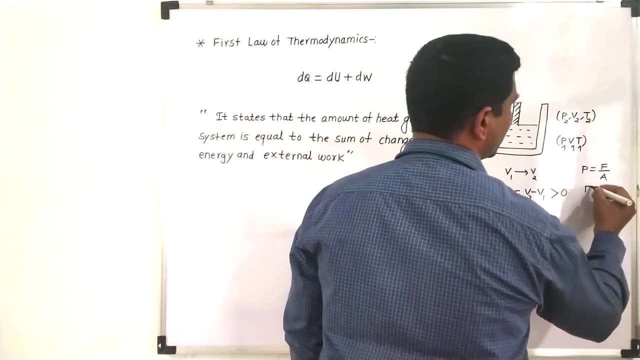 And this piston is displacing with a certain distance. So, and we know that pressure is nothing but pressure is nothing but force upon area, Force upon area. From this one, if I calculate pressure force then it will be Pressure into area. 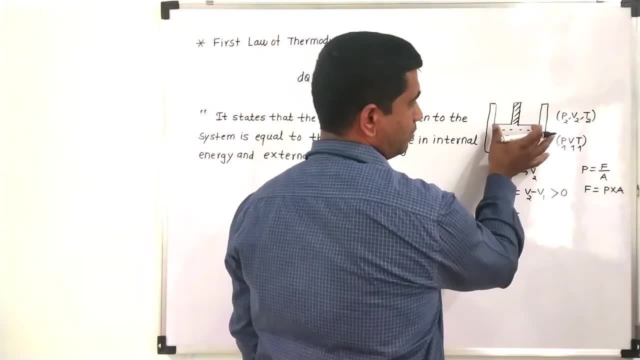 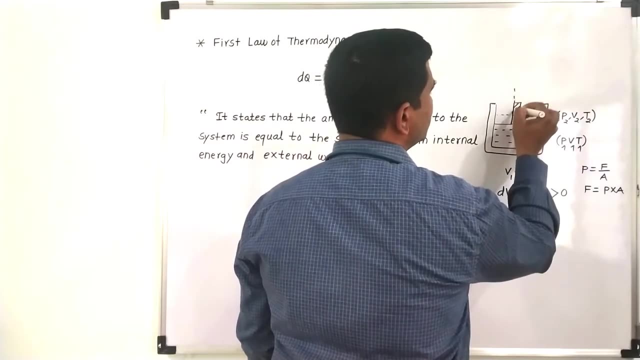 So if I consider A is the area of this piston, And let us say from V1 to V2, let us say this piston is moving from this point to this point. Suppose it is going up to this point. Okay, So this will be the position initial. 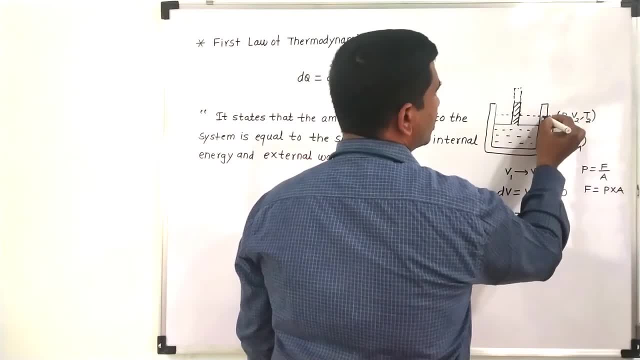 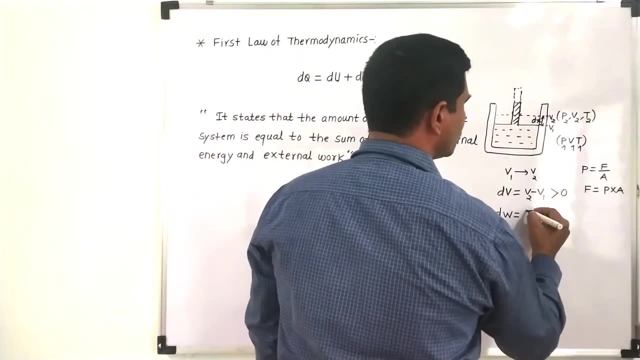 This was the volume V1.. And this is the volume V2.. Okay, So let us say that this is the distance which is covered by this piston. Then my whole thing, it will be force into displacement, which is F into D. 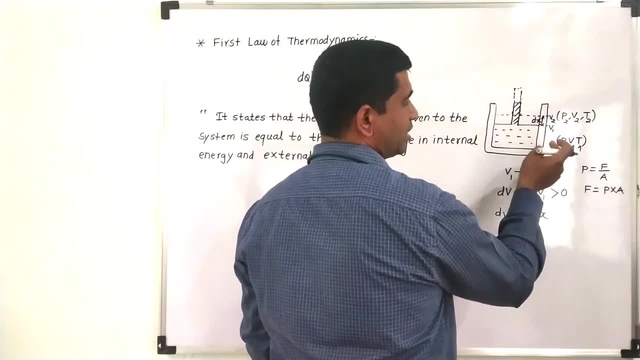 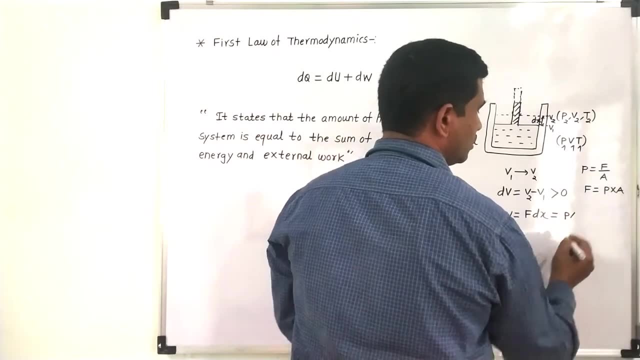 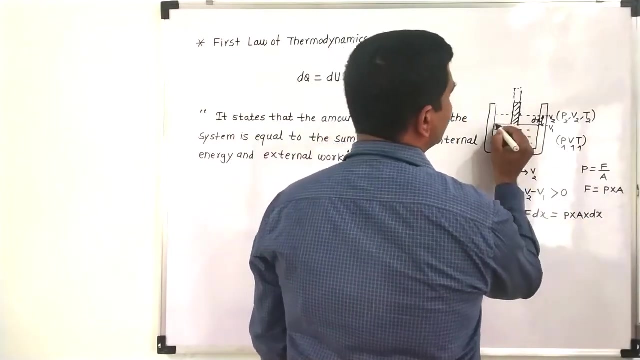 So, whatever the force it will be exerted by this gas on this piston- And we have calculated that force is nothing but pressure into area. Pressure into area, So, and into displacement, that is DX. So area into displacement. If I say that A is the area of this one and this is the displacement, it is a DX. 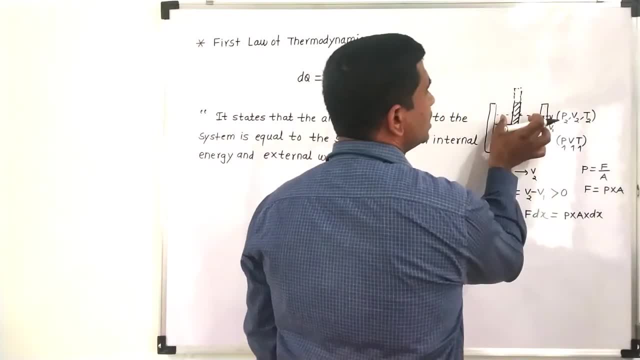 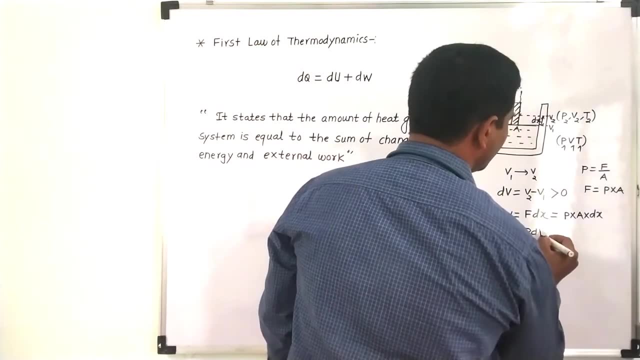 So it is an area multiplied by the height. It is nothing but the volume of this region. And what is this? that volume? That is nothing but the DV change in volume. So it is now going down. It is: DW is equal to P into D. 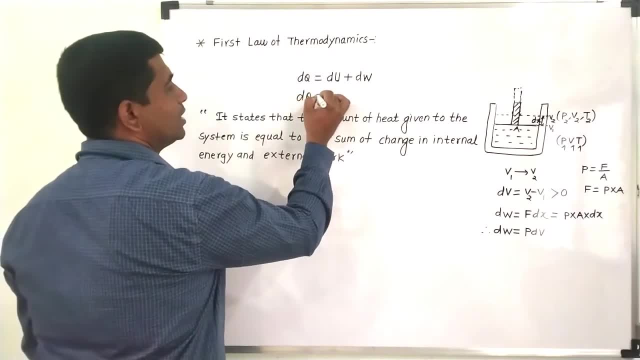 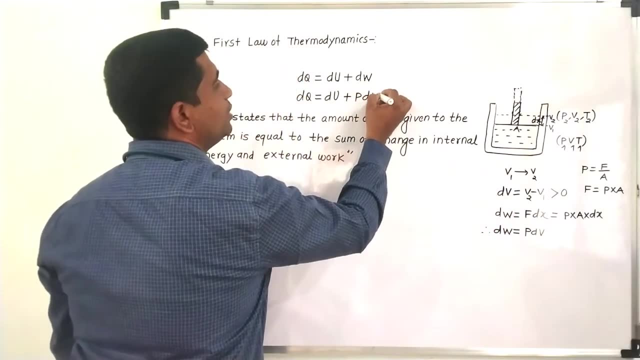 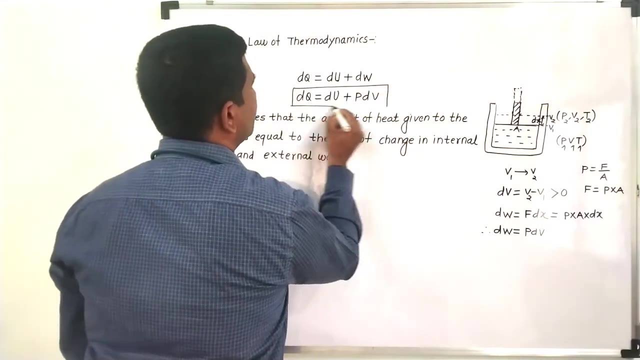 So so this first law of thermodynamics, you can express it in this form as well. Your DQ is equal to DU plus DW. We can rewrite this as a P into change in volume, That is D. So this is nothing but the mathematical statement of the first law of thermodynamics. 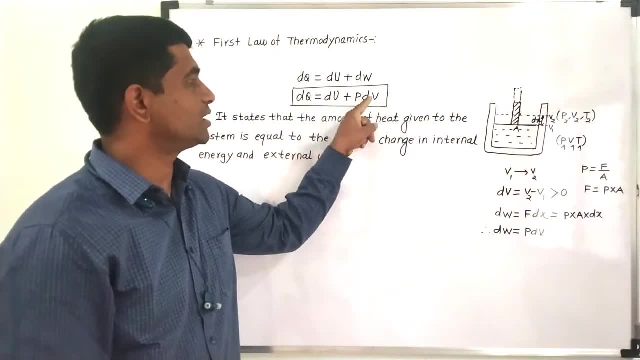 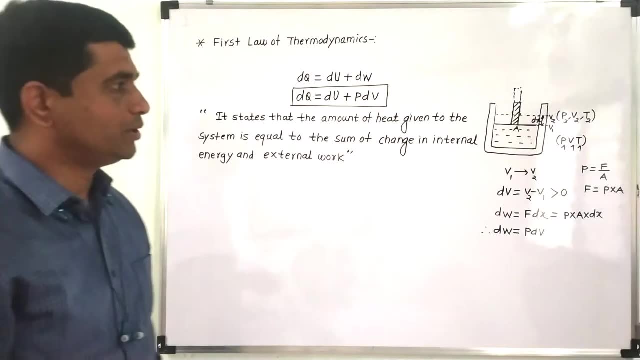 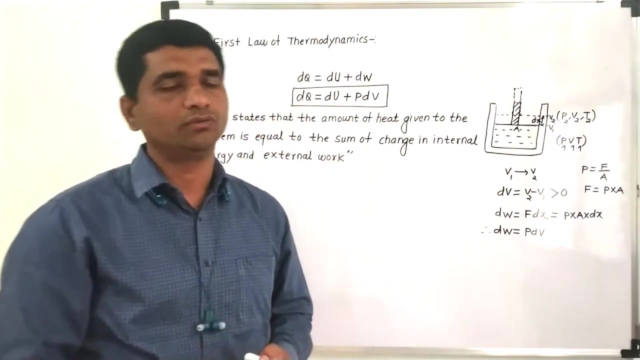 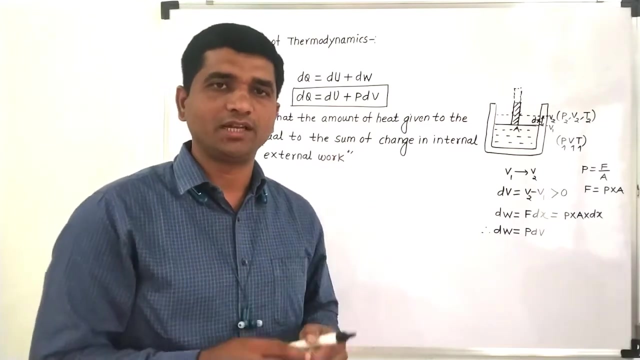 In which the first quantity represents The internal energy, Second quantity represents a work done. Okay, So that is the first law of thermodynamics. Now what we will be doing? we will be considering a different kinds of a thermodynamic processes. Basically, there will be four to five thermodynamic process are there which are very important as far as the engine working of an engine is considered. 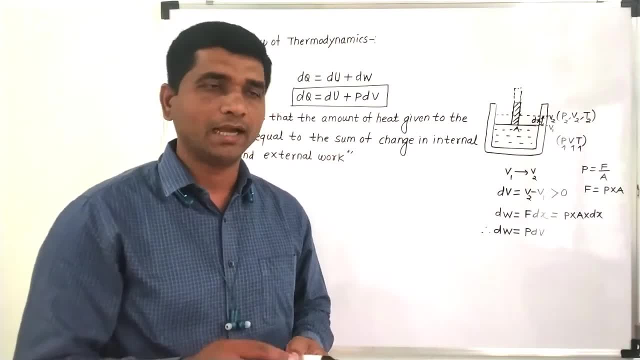 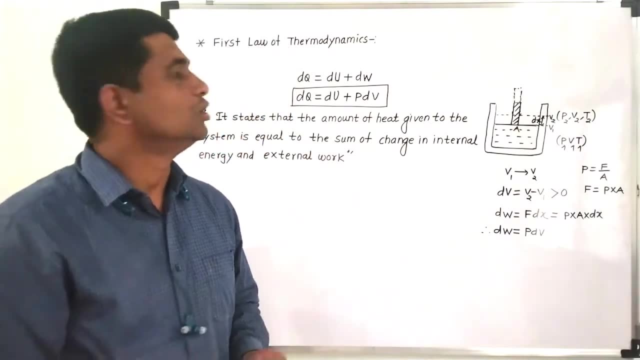 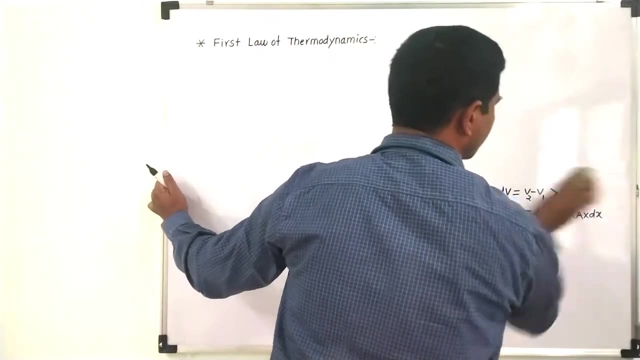 Okay, So those thermodynamic processes we will discuss and we will see how this Wow, First law of thermodynamics behave in those type of thermodynamic processes. So let us start with the next topic. That is nothing but the thermodynamic processes. different thermodynamic processes. 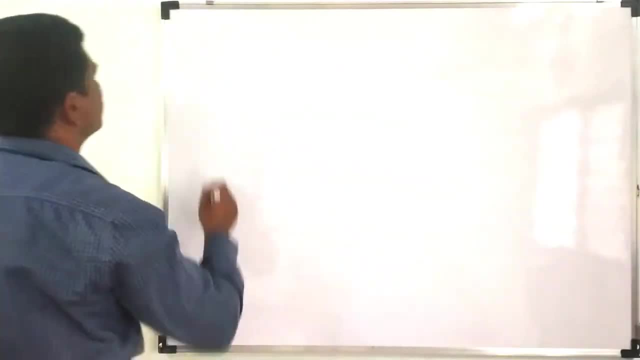 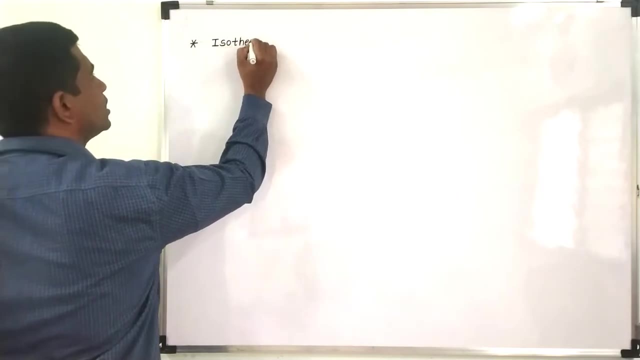 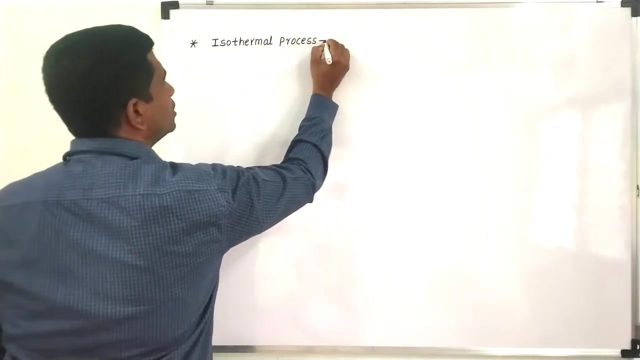 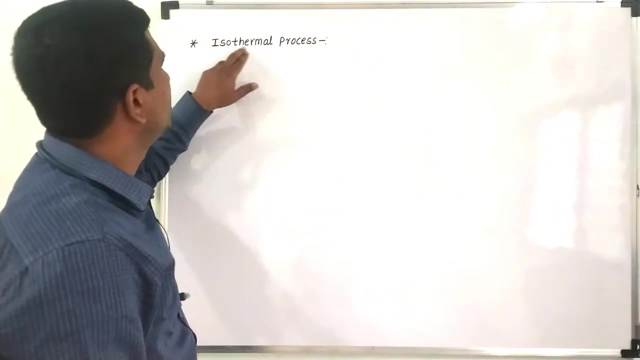 Okay, So first thermodynamic process, it is that that is called as an isothermal process. First of the thermodynamic process, it is that that is nothing but the isothermal process. Isothermal process, Now, what is isothermal? it is derived from the two words, that is iso. iso means same and thermal means temperature. 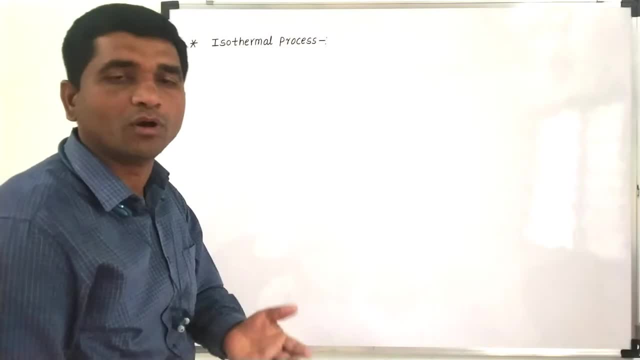 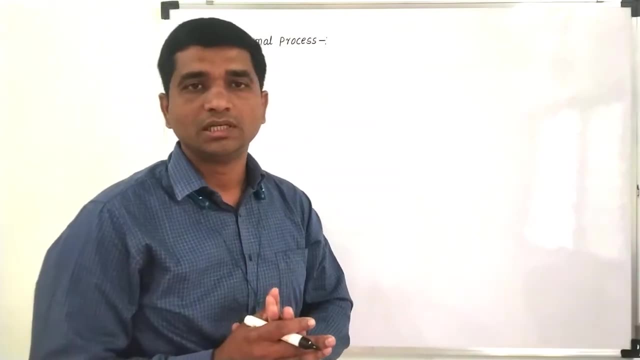 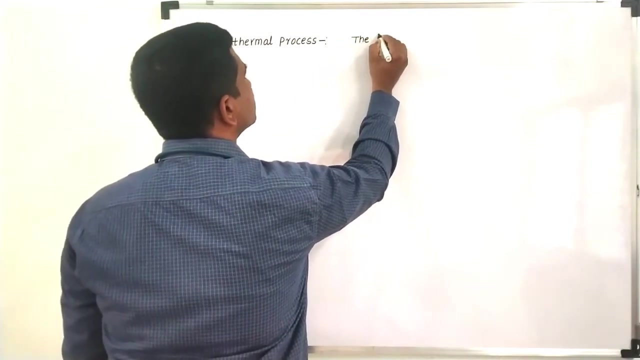 So within the process, if the temperature is remaining same or if some quantity is remaining same as it is constant quantity, So in isothermal process temperature of the system remains constant. So we can define this isothermal process the thermodynamic process, the thermodynamic process. 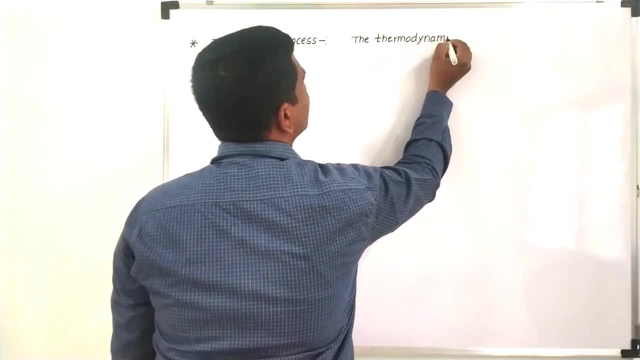 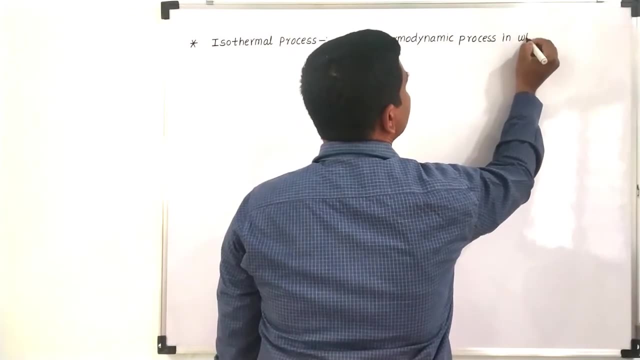 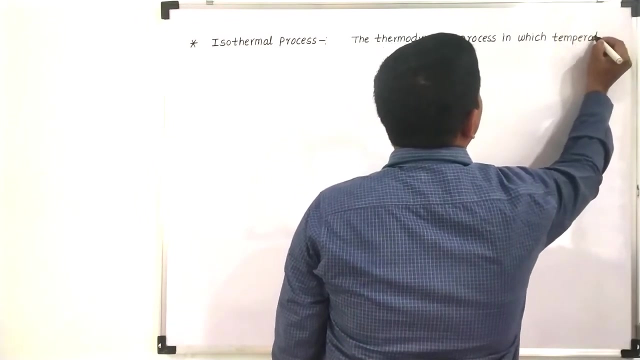 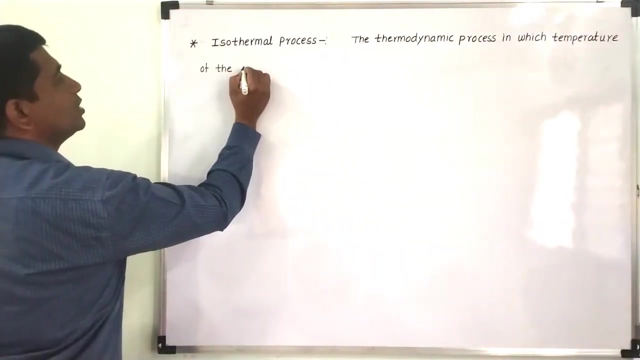 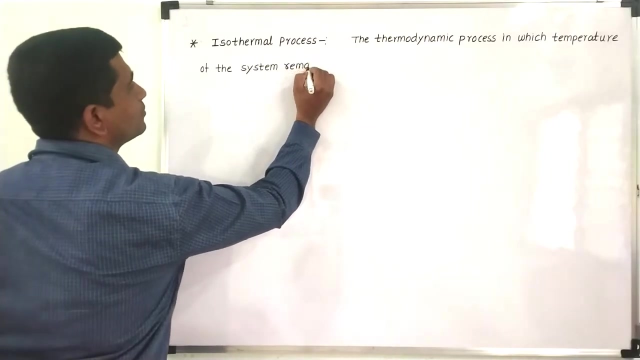 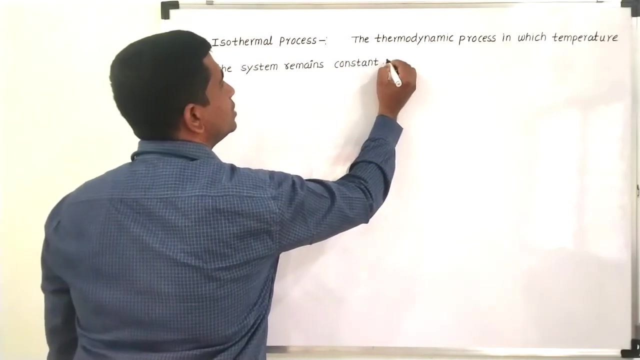 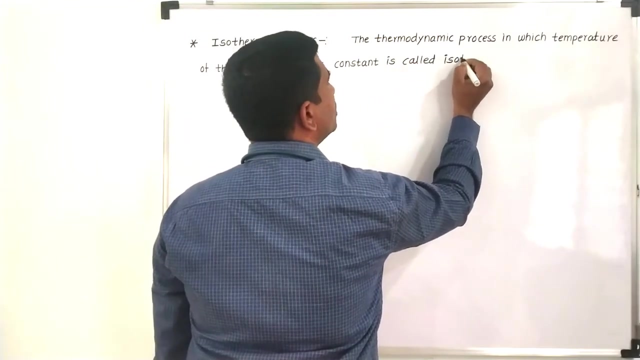 Thermodynamic process in which temperature, in which temperature of the system, temperature of the system remains constant, Temperature of the system, Temperature of the system, Temperature of the system Revenants constant, is called isothermal process. It is called isothermal process. 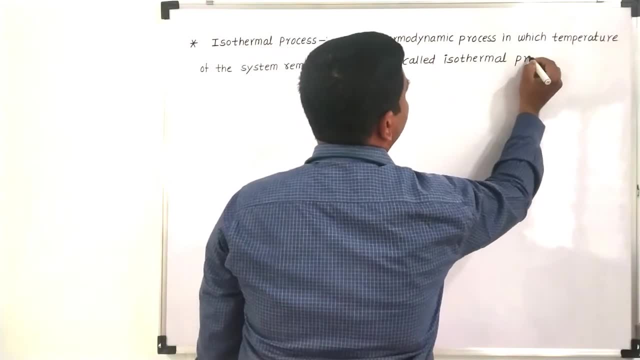 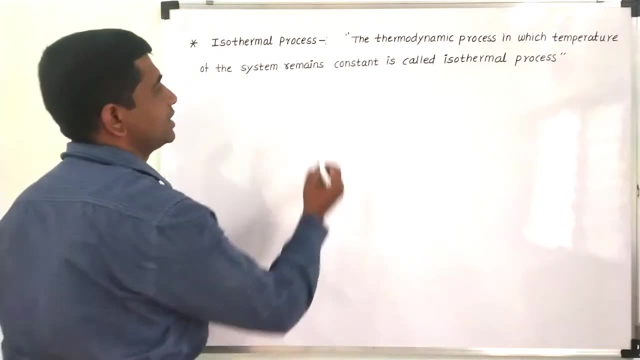 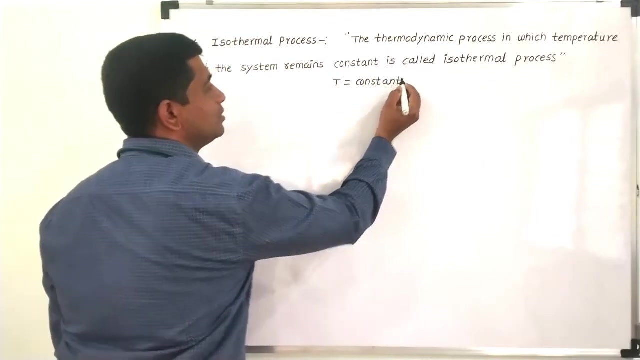 It is called isothermal process. Okay, So that is the definition of an isothermal process. So in this case our temperature is constant. Okay, Temperature is constant. So just in the previous session section we have considered that internal energy. 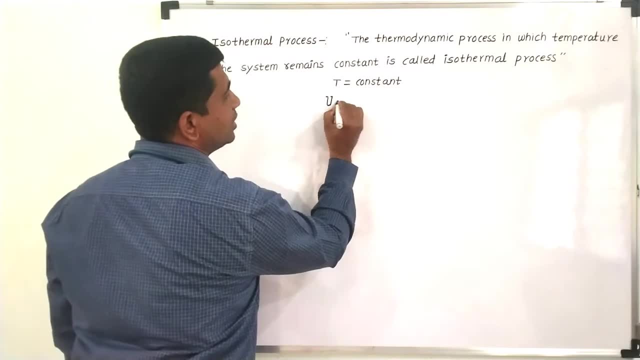 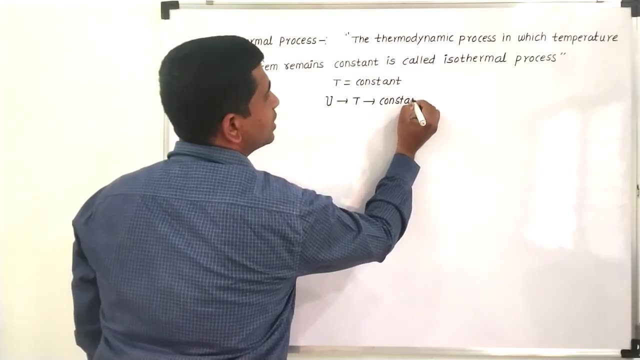 What Internal energy. It is a function of. internal energy is a function of temperature. Now, in this case, as the temperature is constant, as in this case temperature is constant, as temperature is constant, so internal energy, which is a function of temperature. 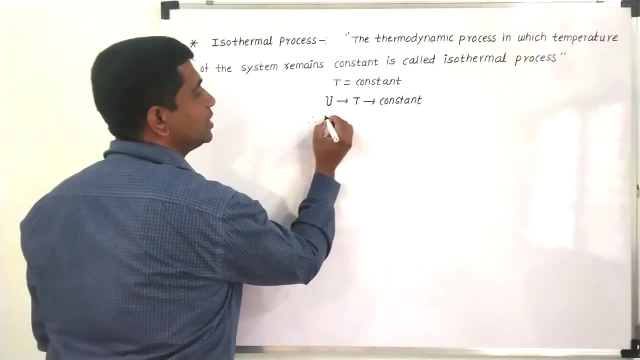 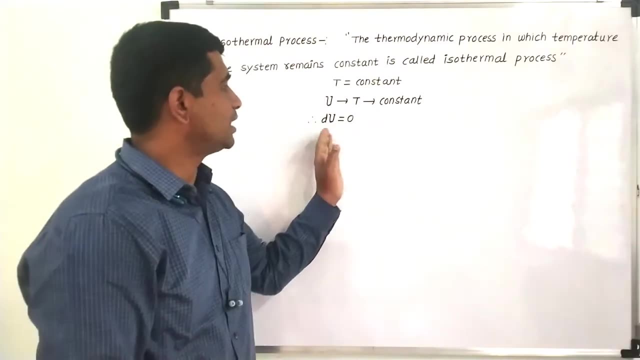 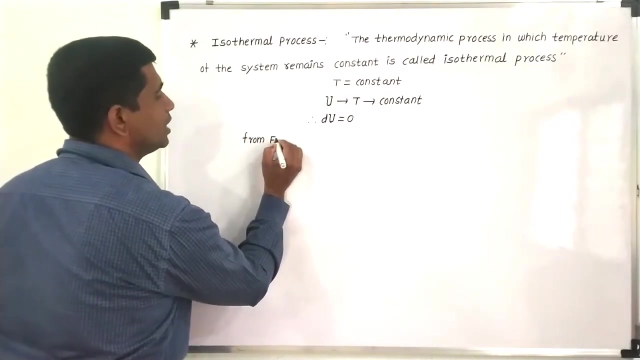 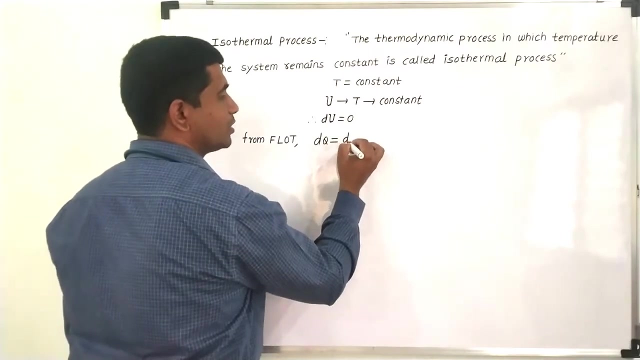 So that will be also constant. And we know that if something is remaining constant, then the change in that quantity it will remain constant. The change in that quantity it will be 0.. So from first law of thermodynamics we know the mathematical statement dq is equal to what is the first law of thermodynamics. 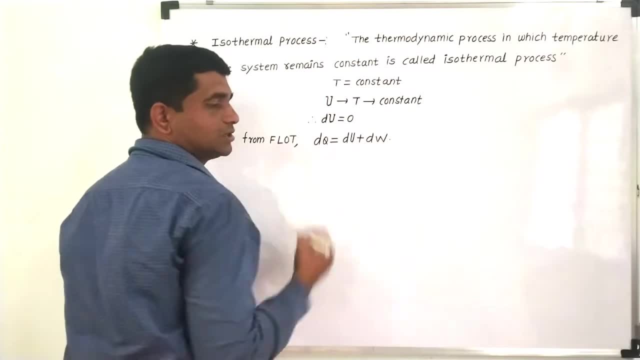 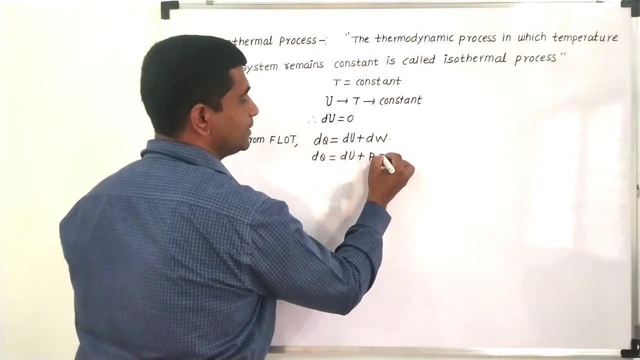 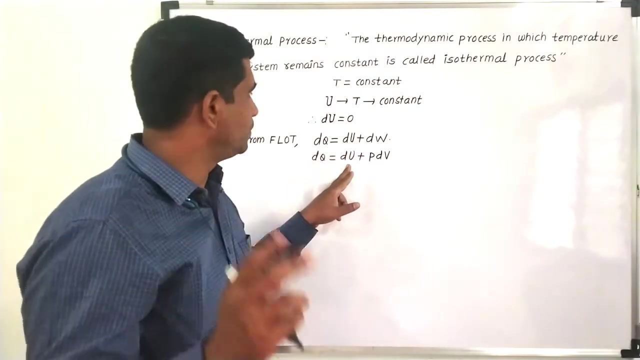 It is du plus dw, du plus dw, And this we can rewrite in this fashion: dq is equal to du plus dw. We have considered that is p into d. So whatever amount of heat is given, it will be utilized for two purposes. 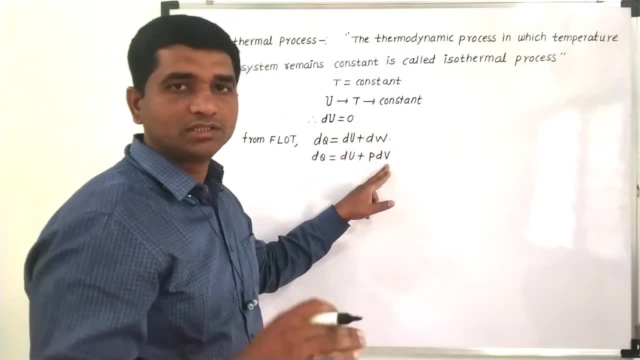 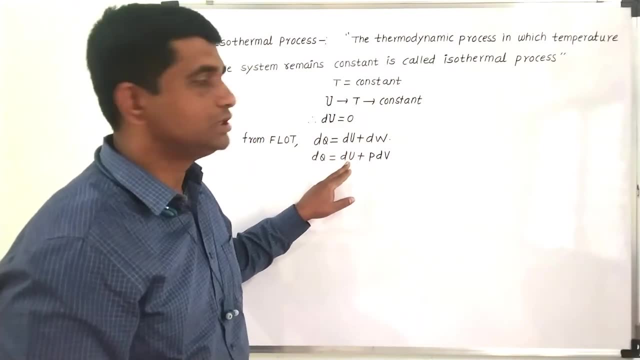 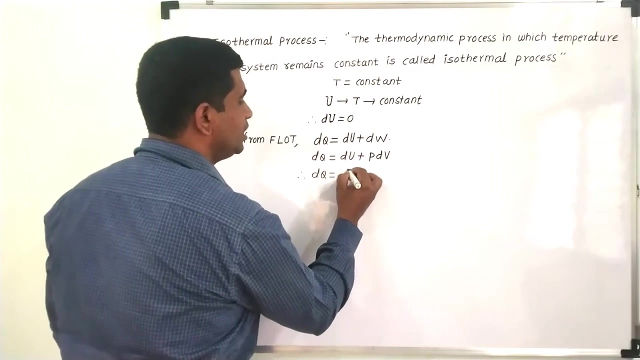 First one is to increase the internal energy and to do some external work. So for isothermal process, as the temperature is constant, so this first term, which is du, it will be 0. So from this one I can rewrite: dq is equal to dw. 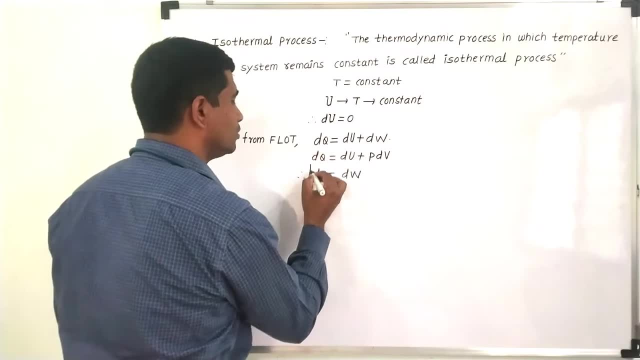 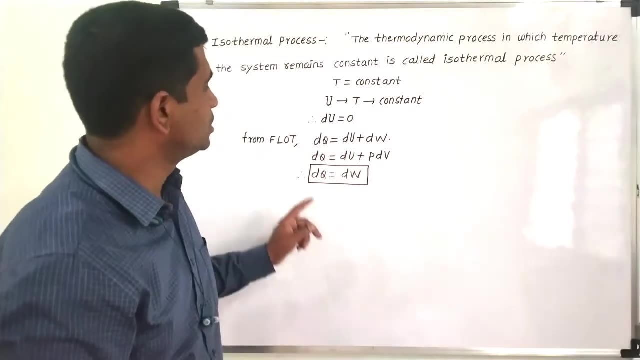 dq is equal to dw, as since du is equal to 0. So from this one we can note it down. In isothermal process, what happens As the temperature is constant? so internal energy is 0.. Change in internal energy is 0.. 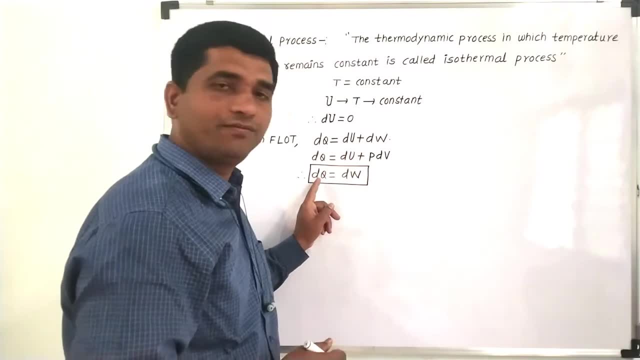 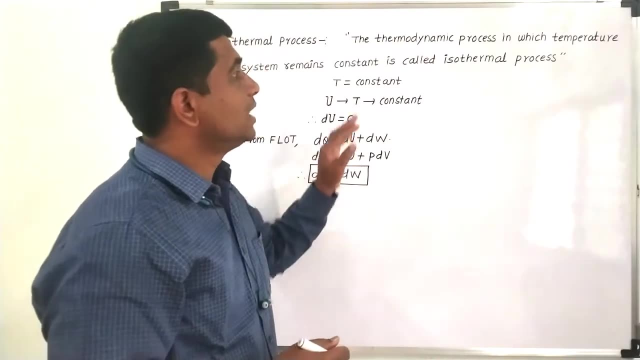 And change in internal energy is 0. So whatever the amount of heat is provided to the system, It will be utilized only for the work done. That is the reason why the maximum work done it will be gained in case of an isothermal process. 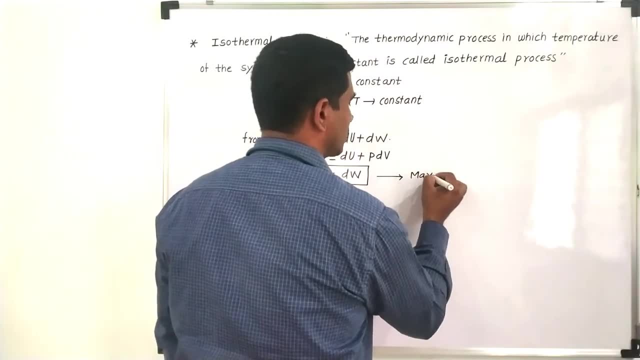 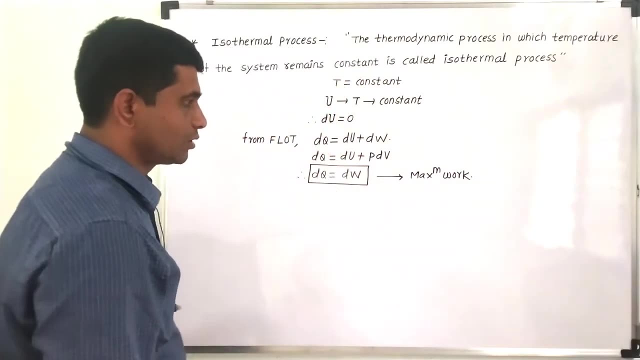 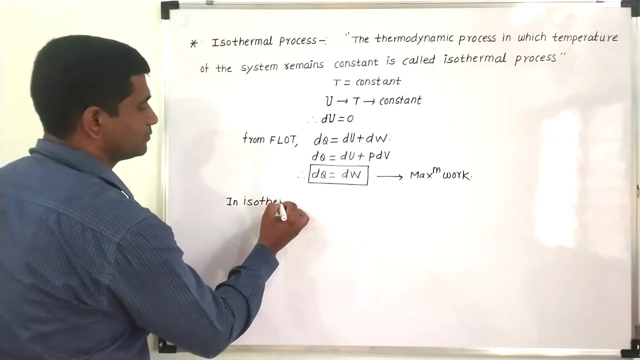 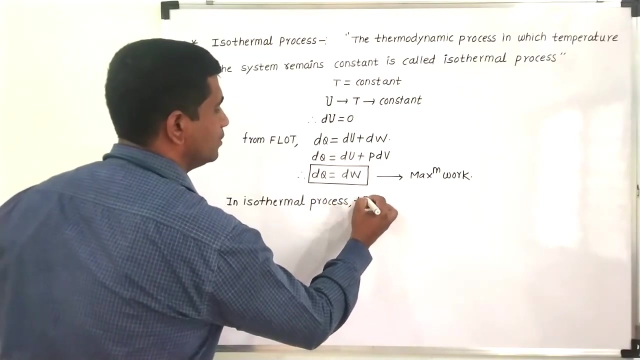 So this is nothing but the maximum work done. Okay, We will be calculating this maximum work done in the next, our next session. Okay, So from this one, in isothermal process, In isothermal process, In isothermal process, the amount of heat, the amount of heat given to the system. 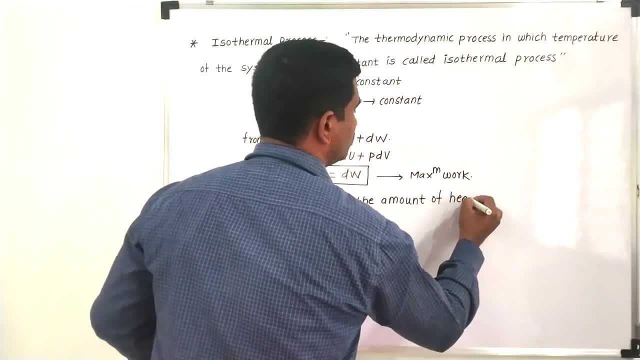 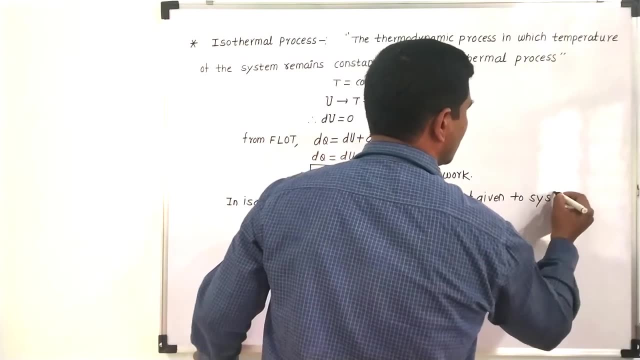 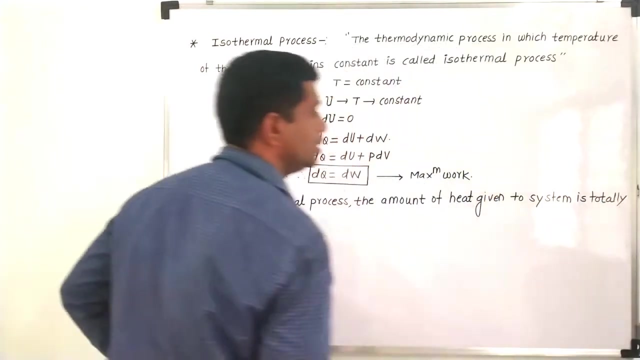 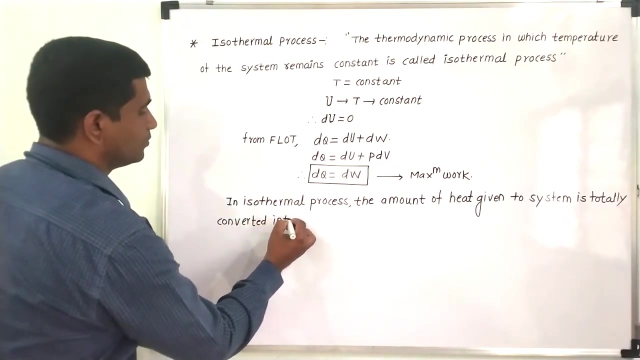 Amount of heat given to the system. Amount of heat given to the system Is: is totally converted into. Is totally converted Into work done. Is totally converted into work done. Okay, So that is why the reason we are getting and maximum work done in this case. 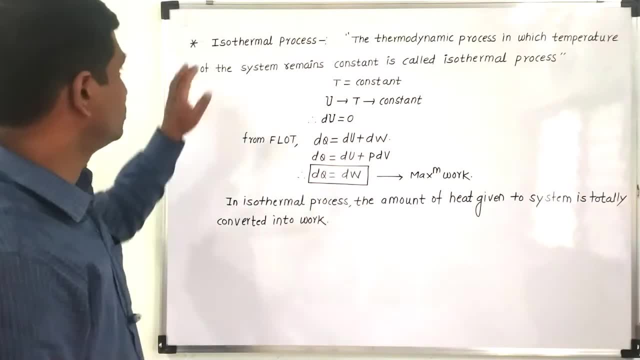 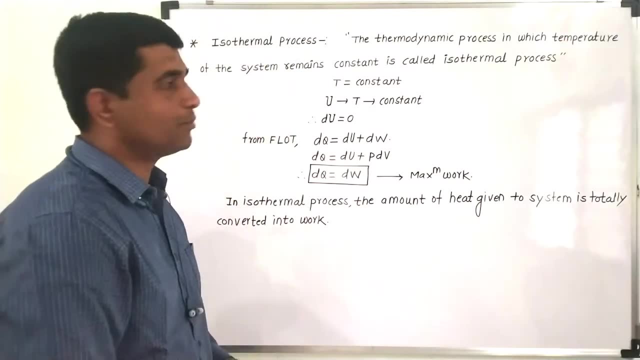 Okay, So that is about the first law of thermodynamics, first law of thermodynamics for the isothermal process. Okay, Now we will move to the next thermodynamics process. that is nothing but the that is called as adiabatic process. 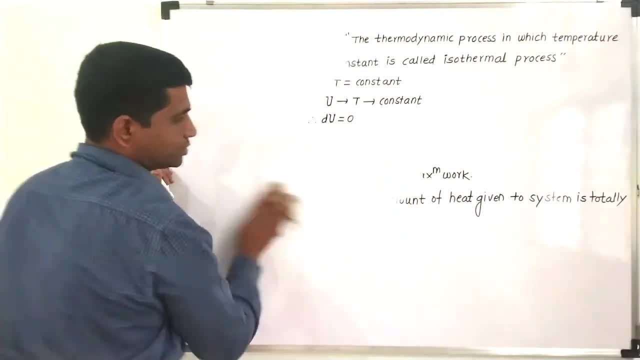 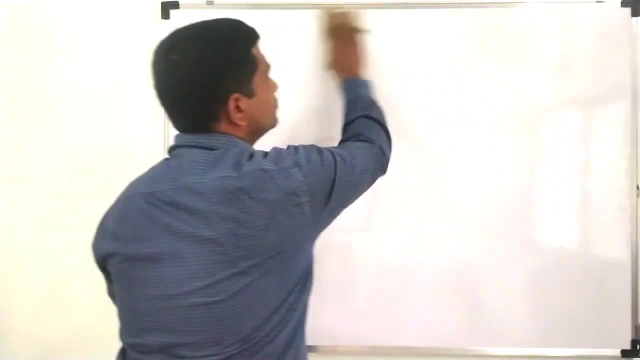 Okay, Now we will consider the adiabatic process. Okay, So let us start with adiabatic process. Okay, Now next thermodynamics cycle, that is adiabatic process. Adiabatic process- Okay. 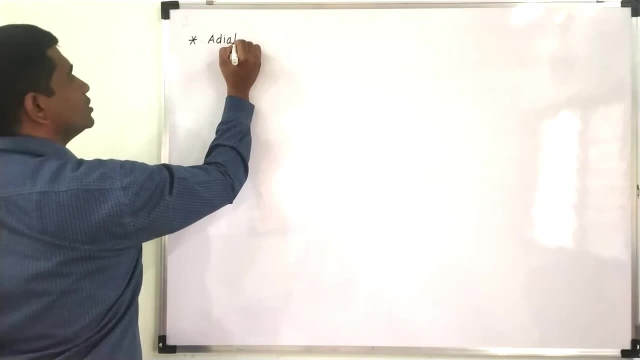 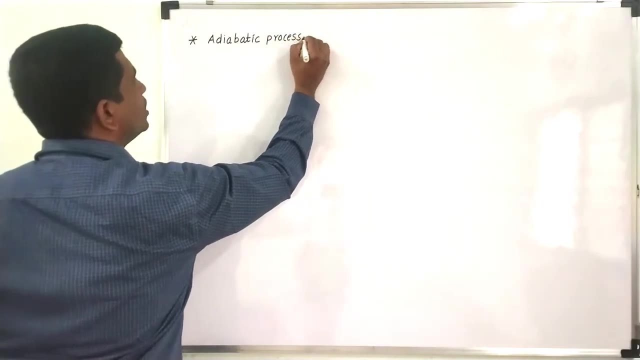 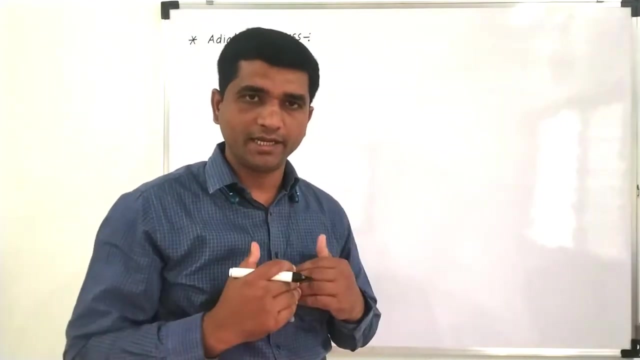 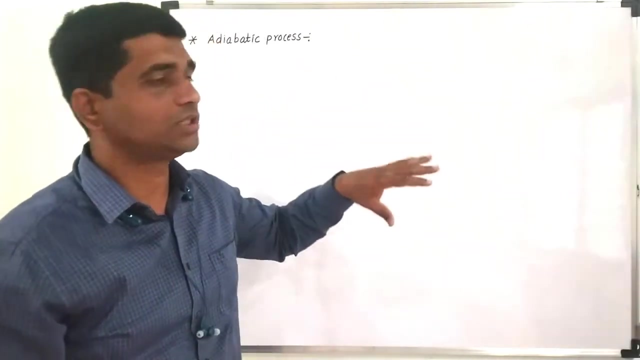 Next thermodynamics cycle. So that is adiabatic process, Adiabatic process. Here I am telling you that adiabatic process is constant return or constantly return, Correct, or it nor gives the heat to the surrounding. ok, so total heat given to the system or taken. 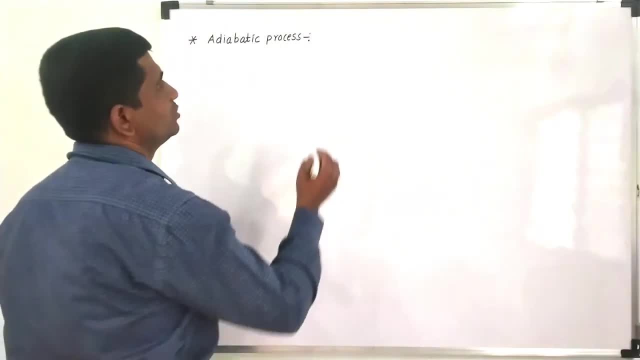 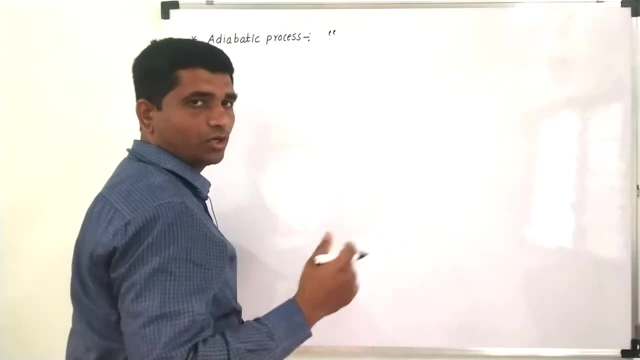 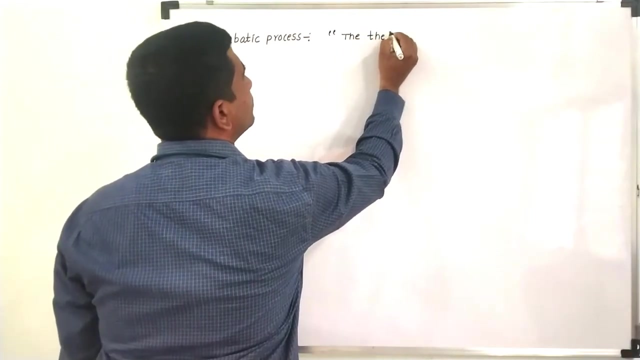 from the system. it is zero. so in this case what we are assuming is that net heat content change in the net heat given to the system or taken from the system- that will be zero. the thermodynamic process, the thermodynamic process, the thermodynamic process, thermodynamic. 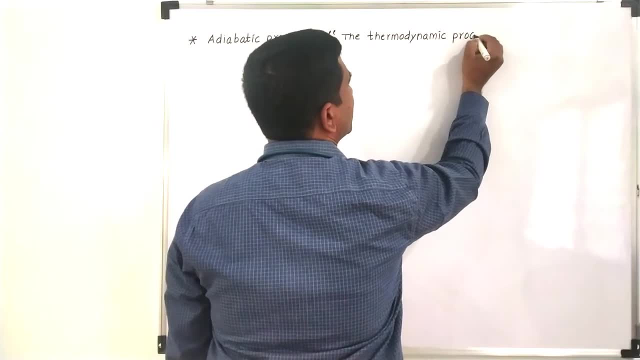 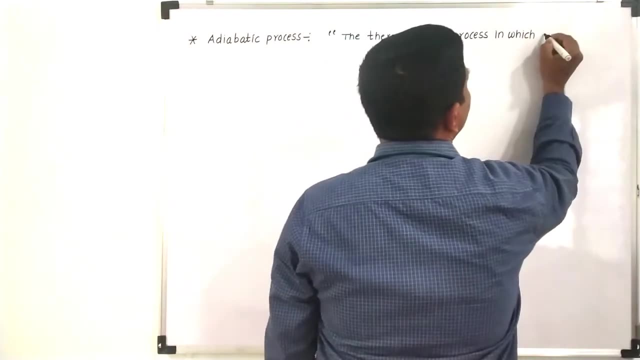 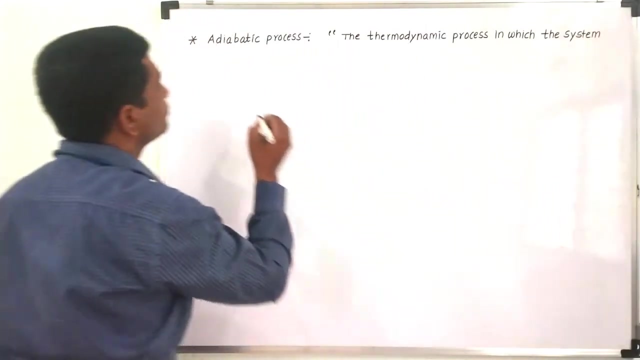 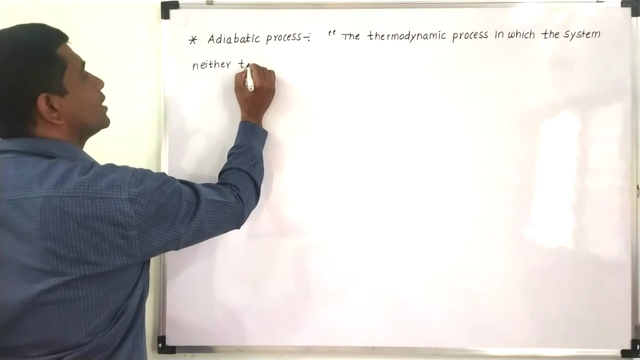 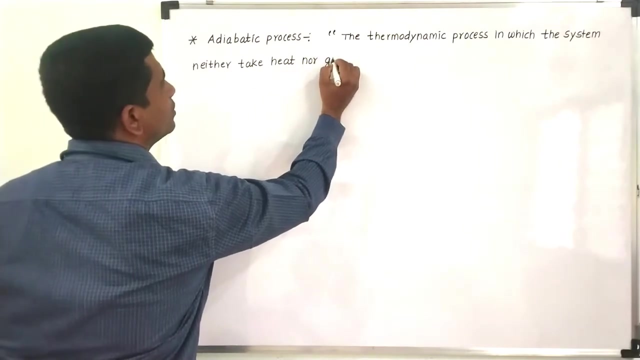 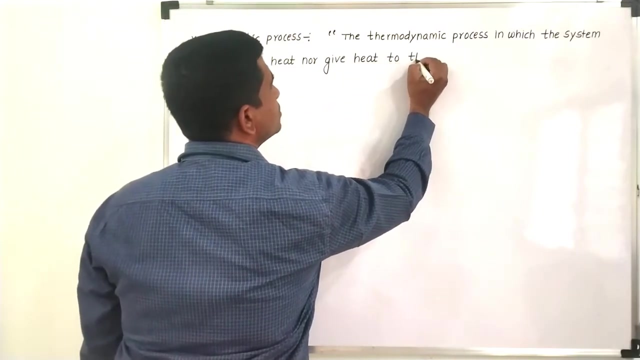 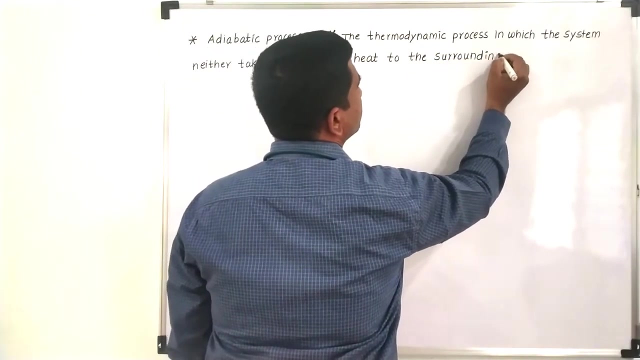 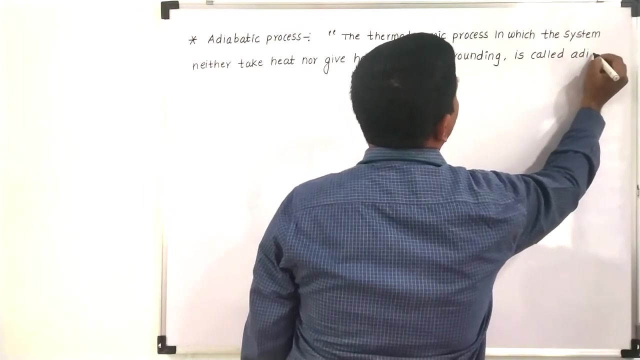 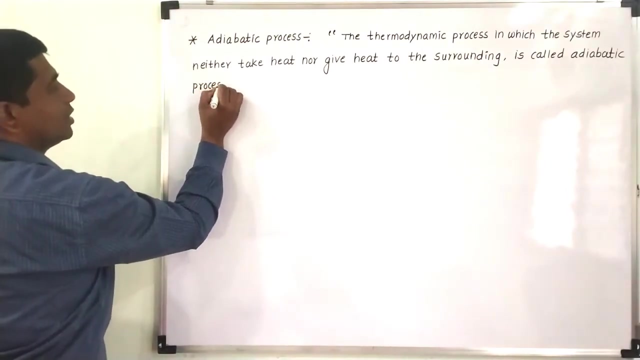 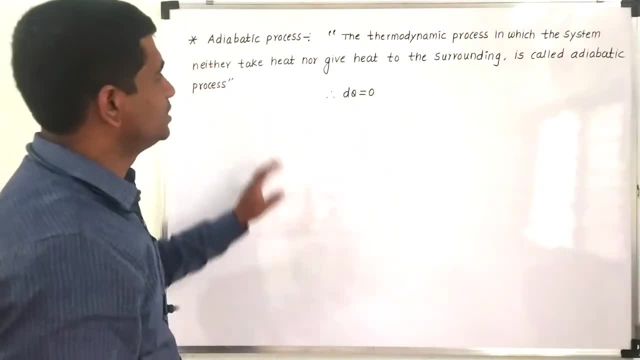 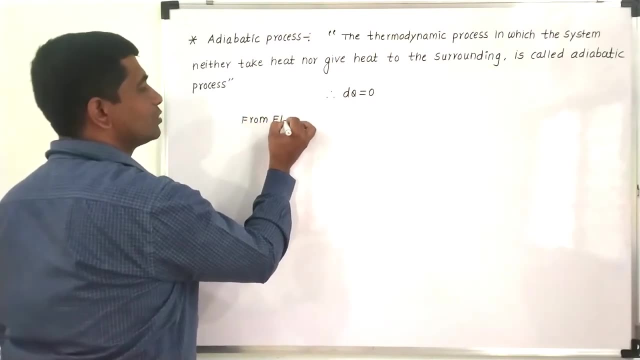 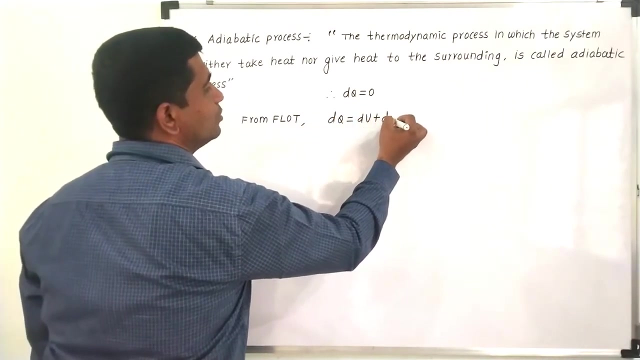 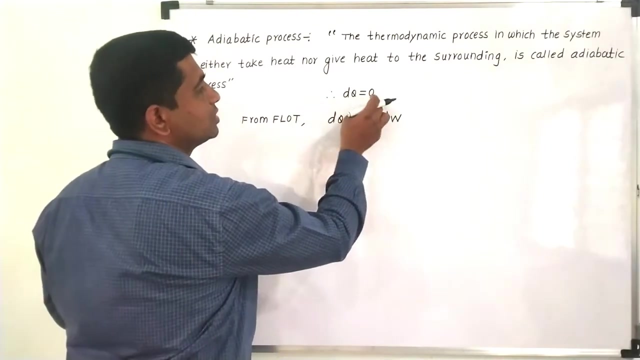 a matter for heat heat, heat heat, thermodynamics. what we have derived is: dQ is equal to dU plus dW. dQ is equal to dU plus dW. that is a mathematical statement of first law of thermodynamics. as for the 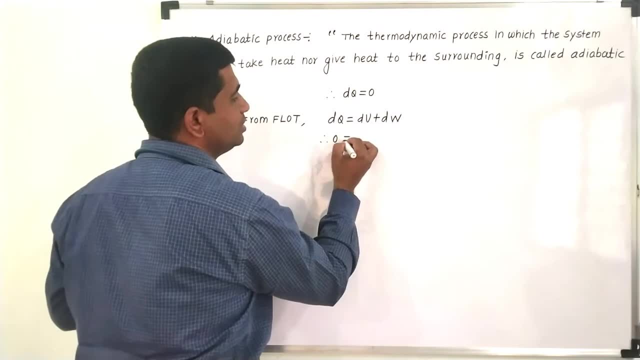 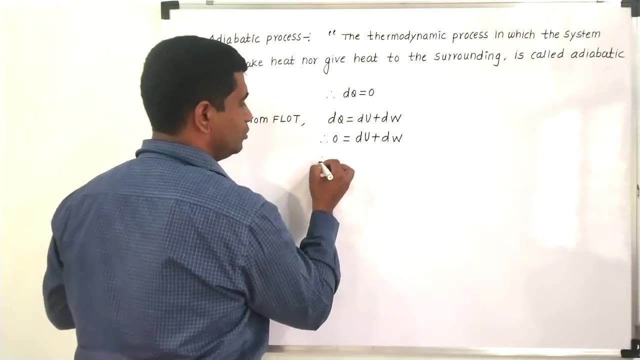 arithmetic questions. dQ is equal to 0,. if I substitute in this equation: okay, dQ is equal to dU plus dW. so dQ is equal to dU plus dW. so from this one I can rewrite dW. 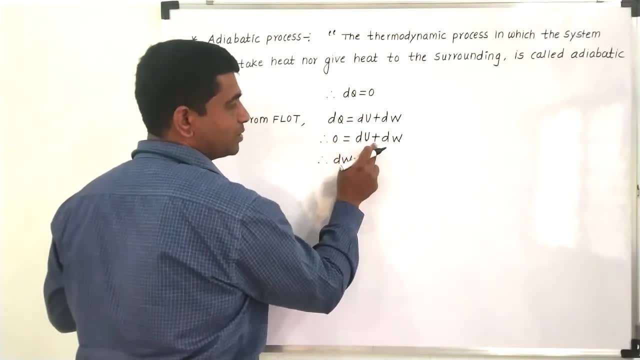 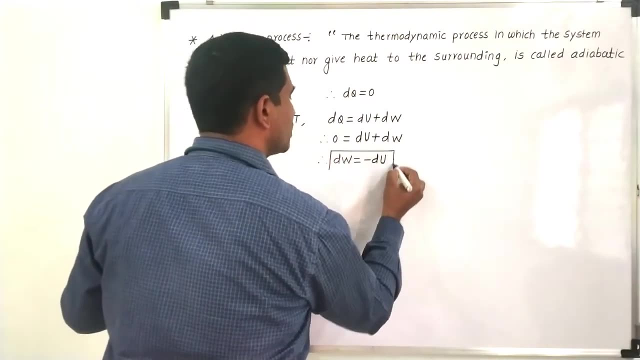 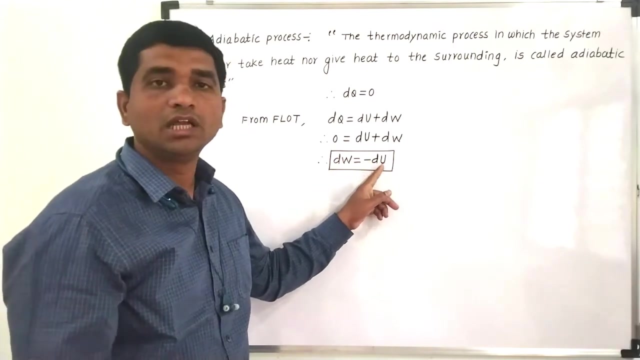 is equal to. if I transfer this dU from this side to this side, it is plus, on this side it will become minus, so dW is equal to minus. dU means so, whatever the amount of work time we will be getting in case of an arithmetic process that will be due to the decrease. 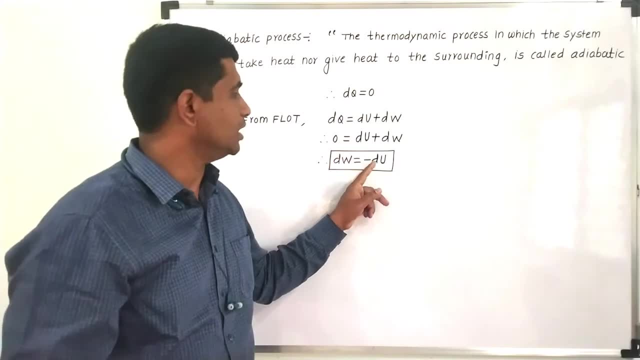 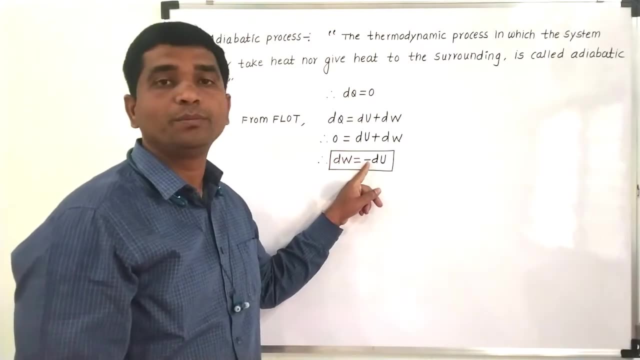 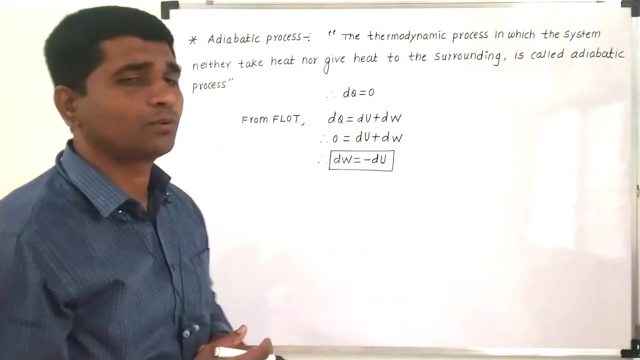 in the internal energy, because here we are getting the negative sign. so change in internal energy will be negative. so final internal energy minus initial internal energy it is coming out to be negative. So it means that the temperature of the system is decreasing. the examples of these processes: 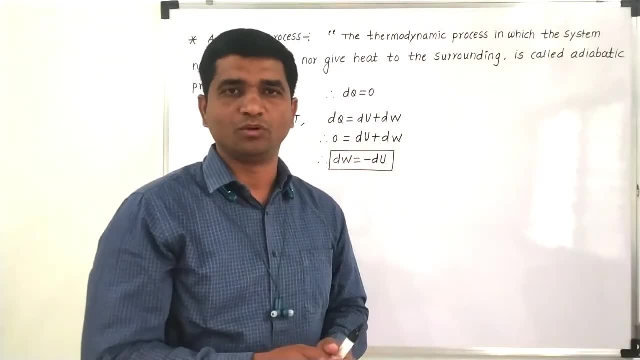 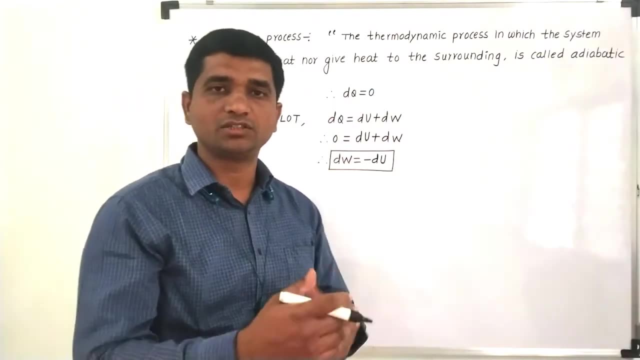 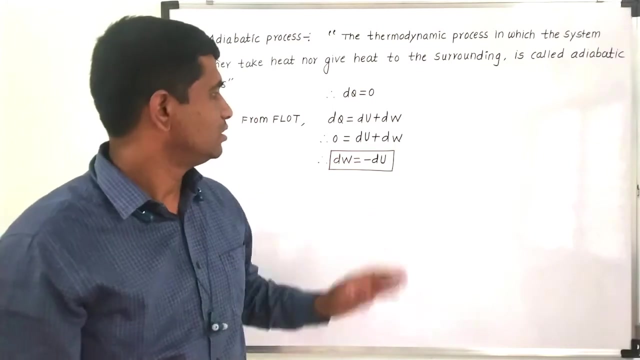 are suddenly, if you puncture the balloon or suddenly a tyre of a vehicle burst, it is an arithmetic process because in this case it is not given to or taken from the surrounding, but suddenly volume decreases or expansion happens. so in that case the 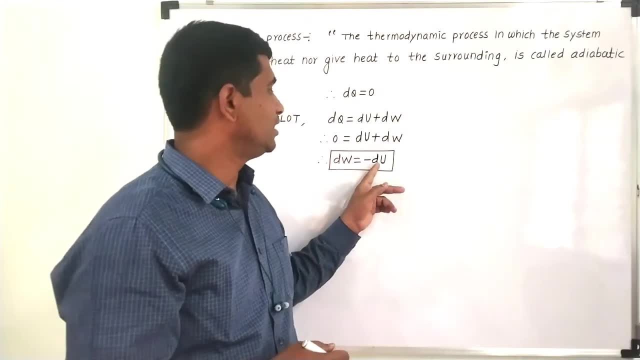 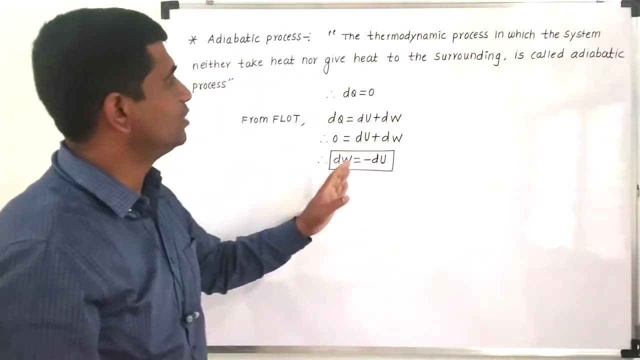 work time which we will be getting. it is due to the expense of the internal energy. due to that one, the temperature of the system falls, means the internal energy decreases. so you can write down from the arithmetic process the amount of work done in arithmetic. 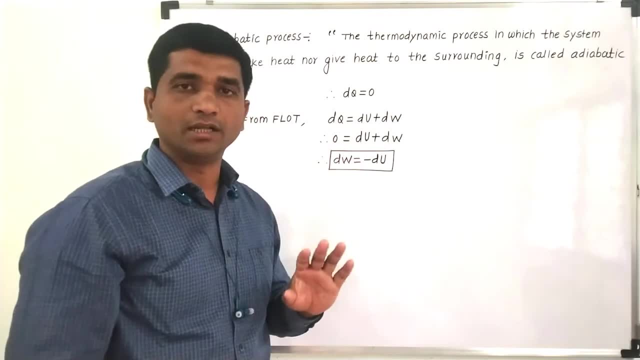 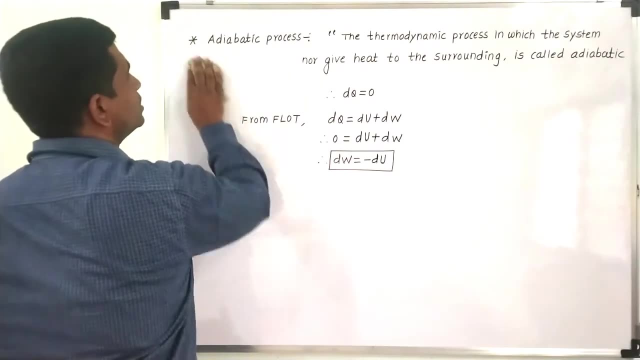 process. it is due to the expense of the internal energy. okay, so that is an arithmetic process. we will consider now the third important process. it is there. that is nothing but isobaric process. third process: it is there, isobaric process. 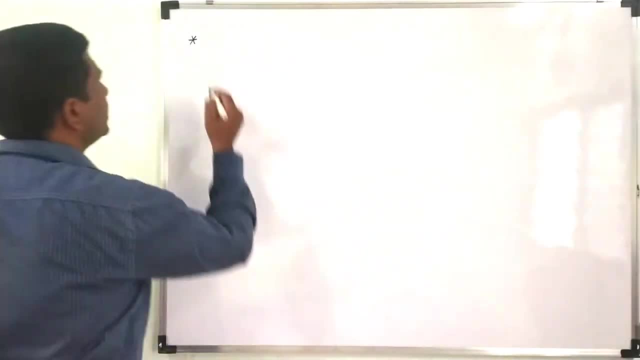 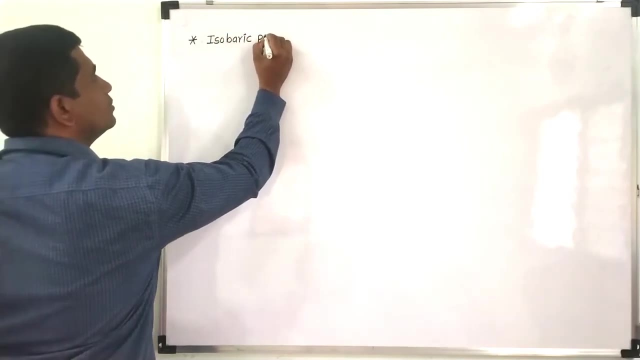 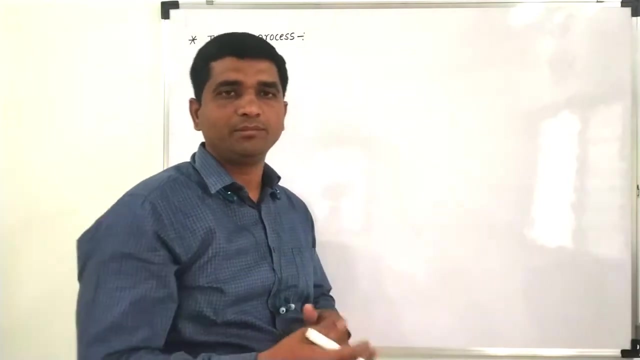 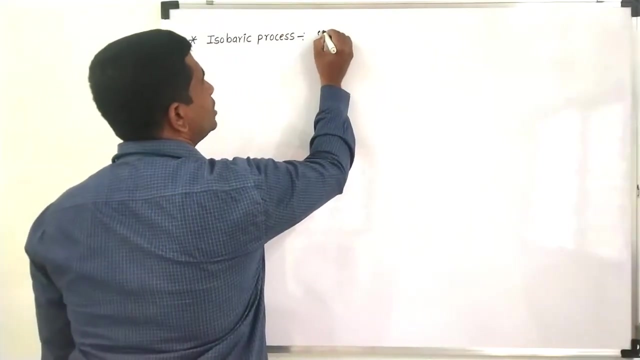 Third process, that is, isobaric process. okay, isobaric process. now what happens in case of an isobaric process, if the thermodynamic change it is occurring at a constant pressure? such a kind of process is called as a isobaric process. so we will note it down: the thermodynamic 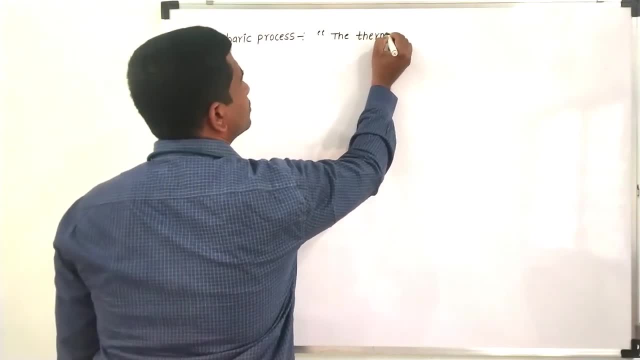 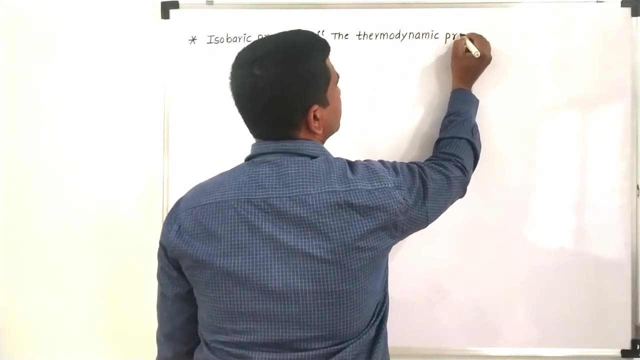 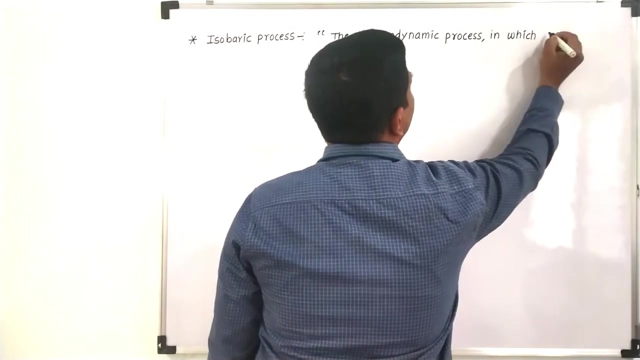 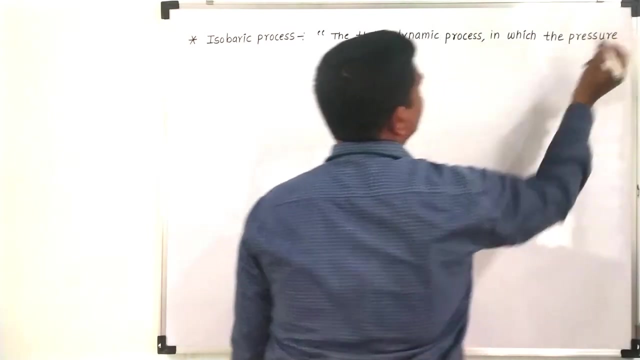 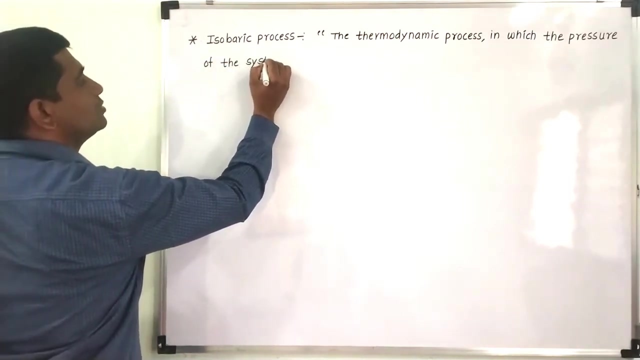 process, the thermodynamic process. Okay, Okay, The thermodynamic process in which the thermodynamic process, in which, in which the pressure, in which the pressure of the system, pressure of the system, pressure of the system remains constant, 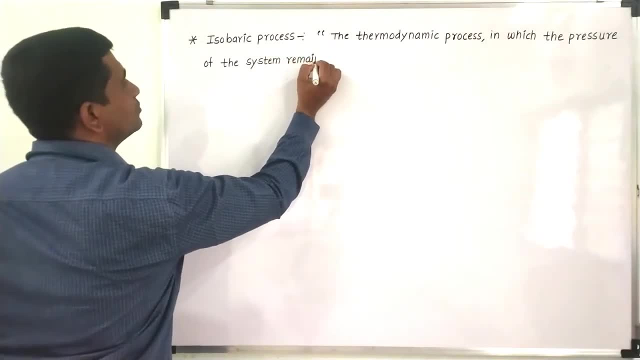 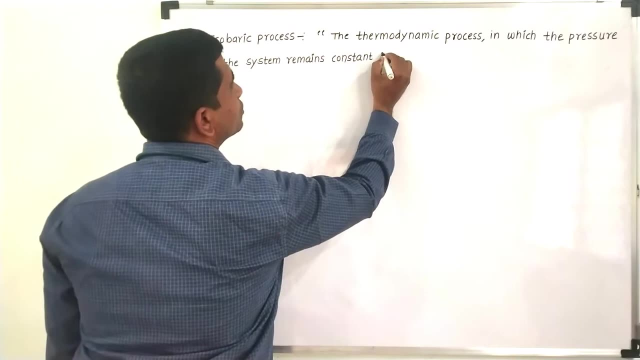 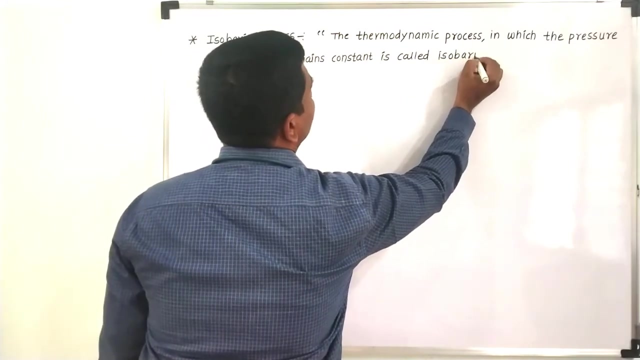 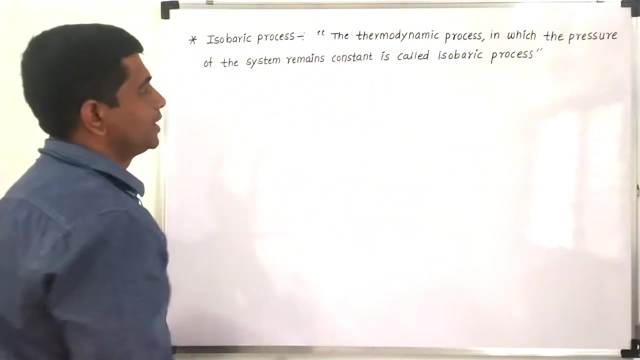 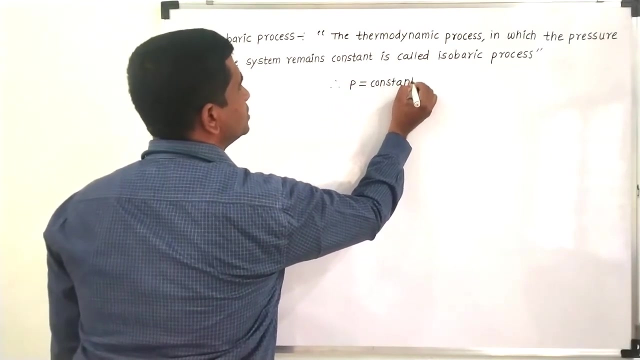 system remains constant. constant is called pressure of the system is constant is called isobaric process, is called isobaric process, is called isobaric process. okay, so for an isobaric process, what we are having? this pressure is equal to constant. pressure is equal to constant. that is that simple limitation. 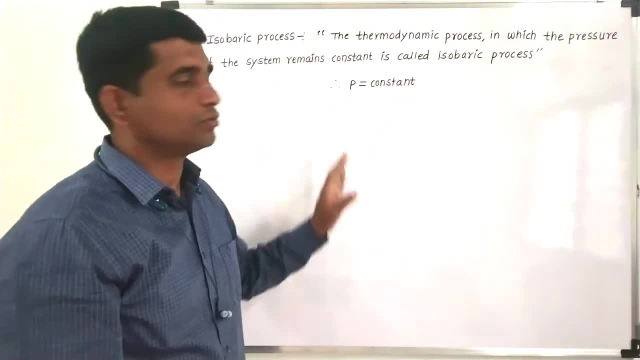 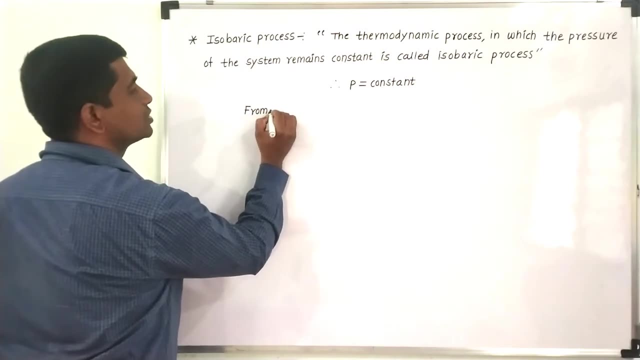 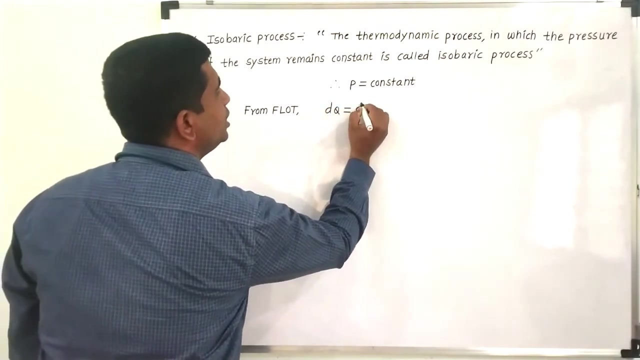 is that pressure during the system it will be constant. pressure during the it is constant from first law of thermodynamics. we will consider what we get from the first law of thermodynamics. from first law of thermodynamics what you can have is: dQ is equal to Du plus Dw. we know that this volume 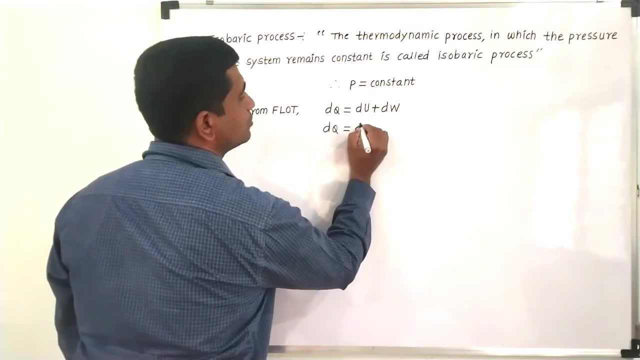 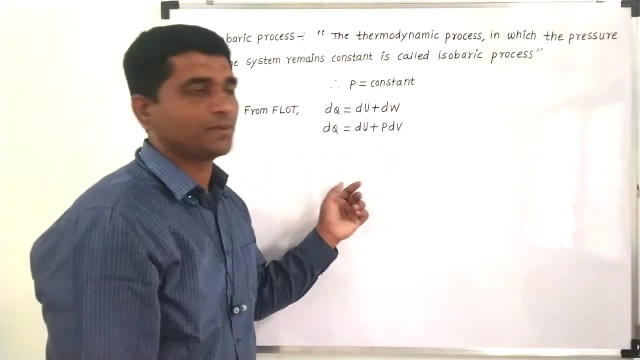 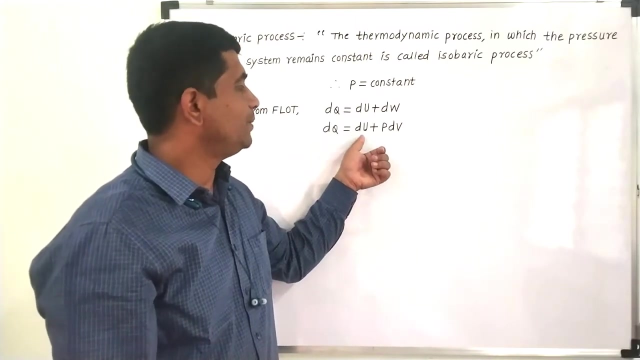 we can rewrite: dq equals du, which is 자� is equal to d, cube is equal to du, plus one term. we can rewrite this as a pd. so if you consider from this expression, in this case pressure is remaining constant. so here the, whatever the amount of heat is given, it will be used for the two purposes. one is for the 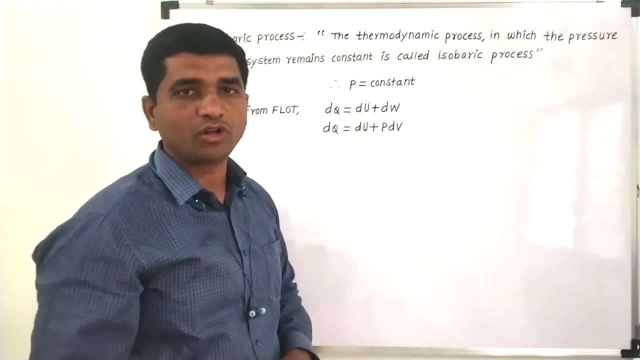 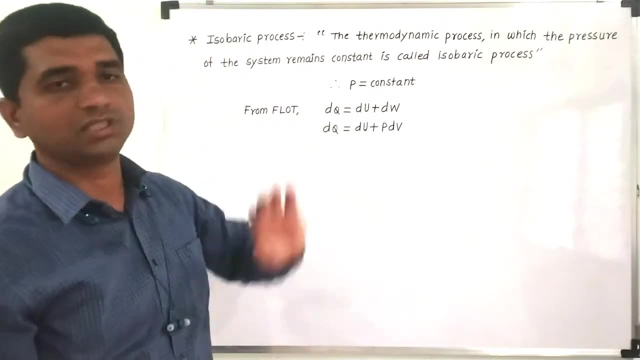 to change its internal energy and to perform some amount of external content. so in this case, the first law of thermodynamics, it is not showing any kind of change in the process it is considered. it is isobaric process and the last, most important process it is there. 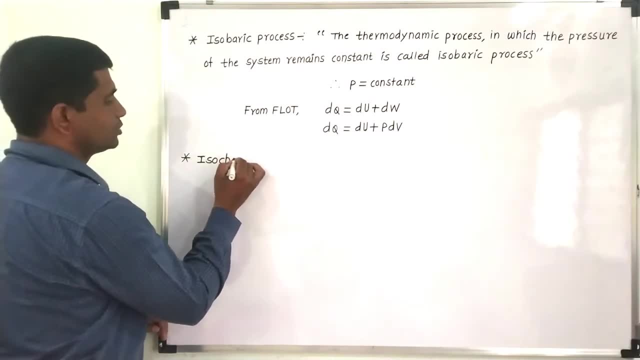 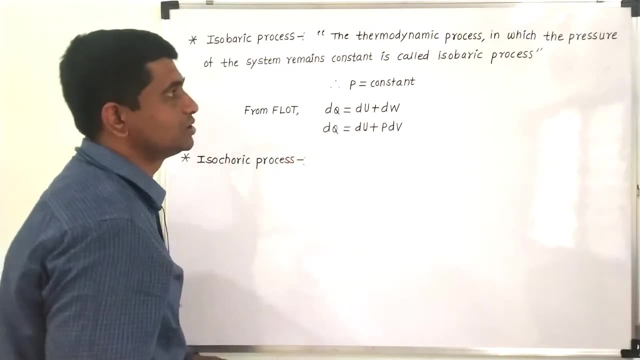 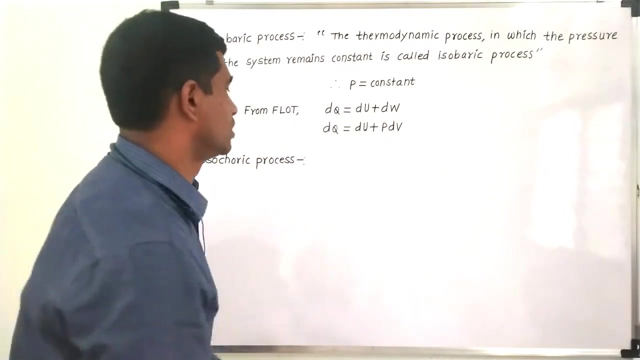 that is called as a isochoric process. the last process, which is of prime importance, that is isochoric process. so what is isochoric process? as in isobaric process, pressure remains constant. in case of isochoric process, volume remains constant. okay, so we will. first of 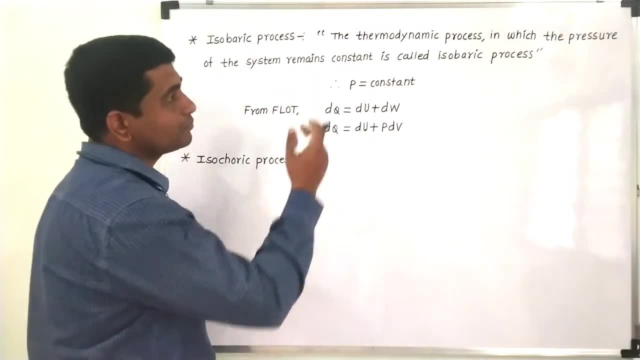 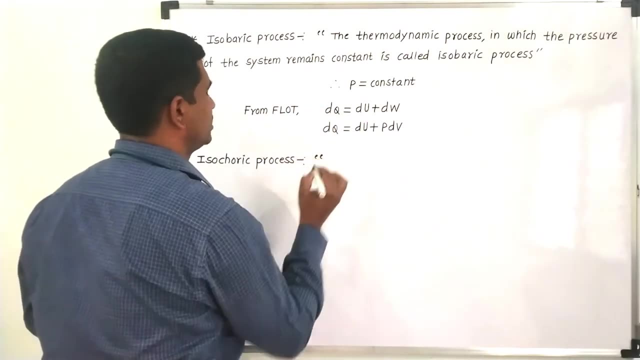 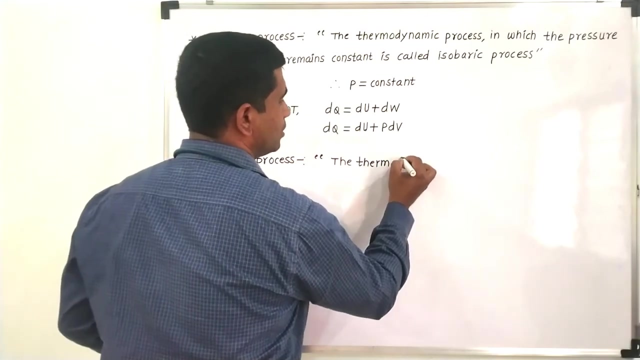 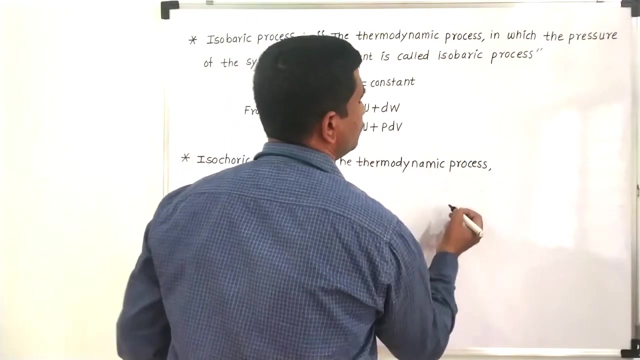 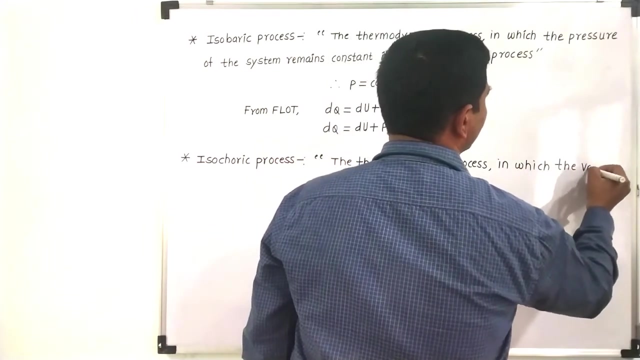 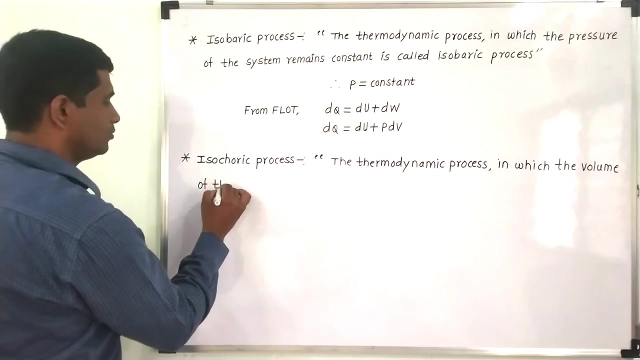 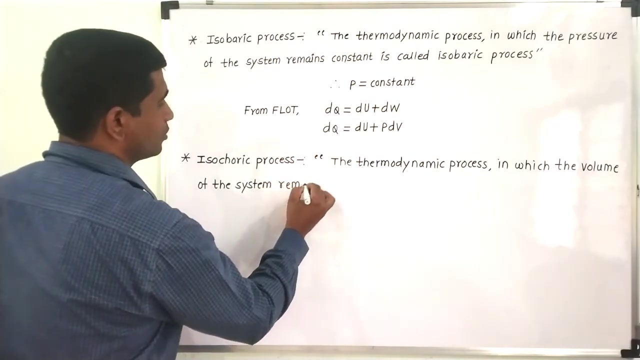 all define this, what is isochoric process? and then we will try to calculate the amount, calculate what significance we can calculate from the first law of thermodynamics, so what it is, states that the thermodynamic process, the thermodynamic process in which the thermodynamic, the thermodynamic process in which the volume of the system remains constant, 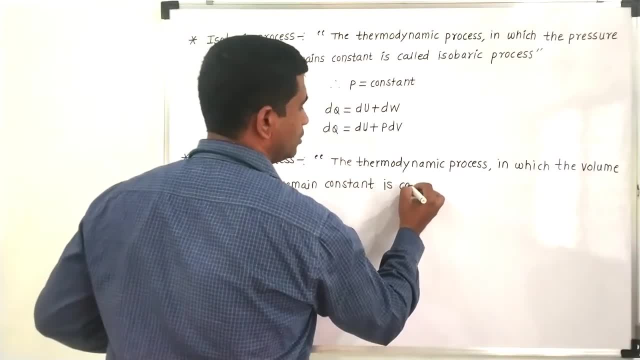 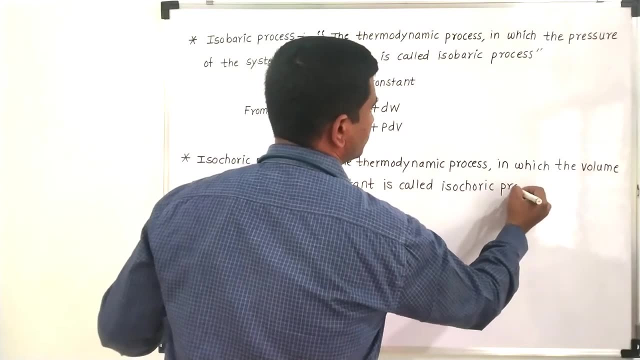 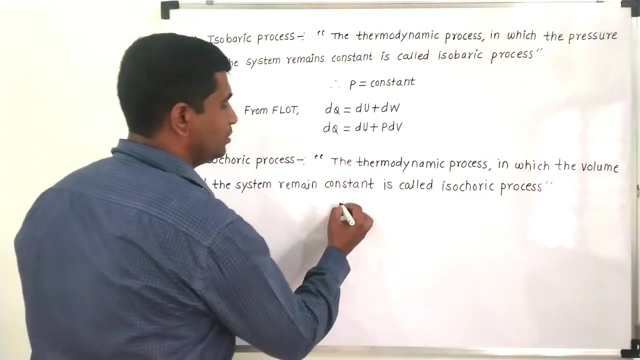 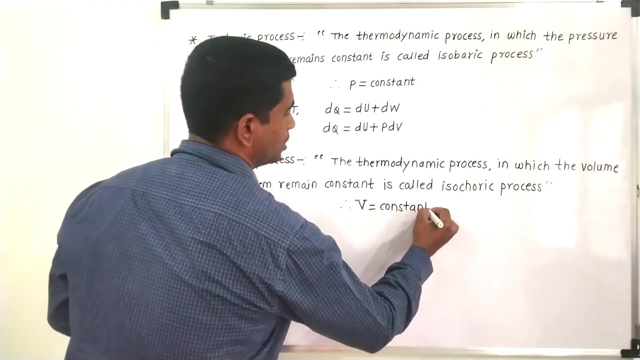 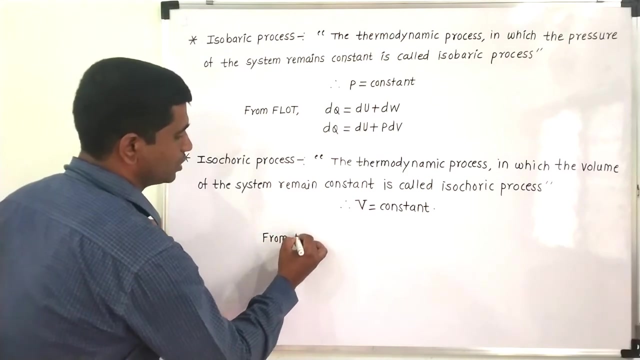 is called isochoric process. so for an isochoric process, volume remains constant. so V is equal to constant. for this isochoric process, volume remains constant as volume is constant. so what happens from the first law of thermodynamics? we know the statement of the first law of thermodynamics. 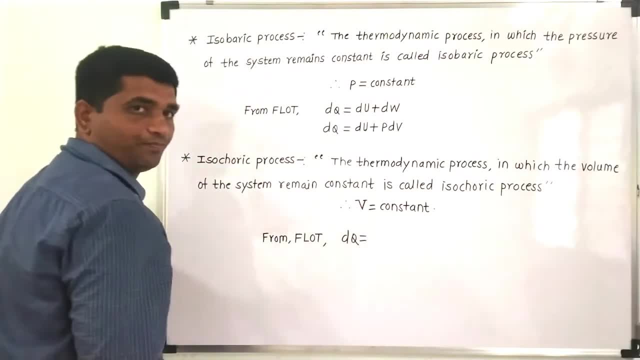 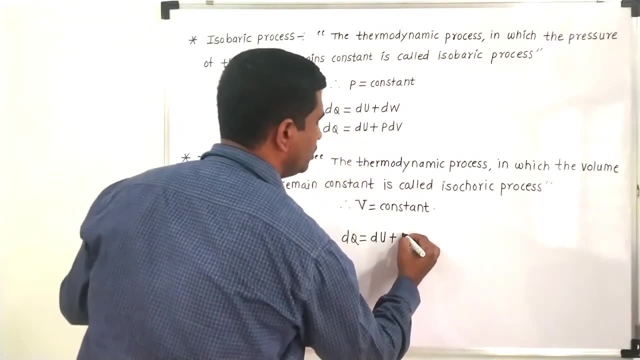 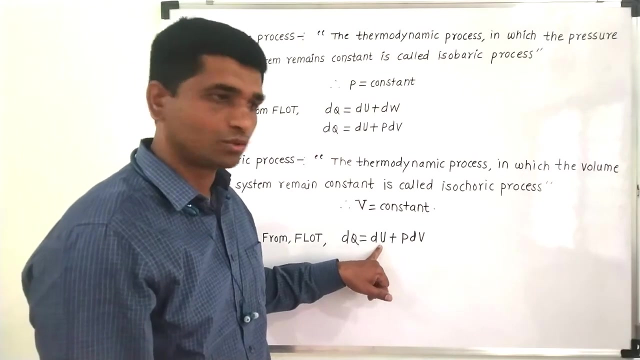 what is first law of thermodynamics: dQ is equal to what is that? dU plus dW. dW is nothing but the P into dV. so whatever the amount of heat it is given, it will be used to increase the internal energy and to perform some external work. 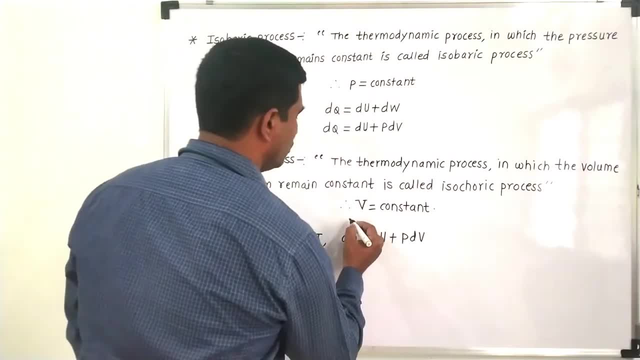 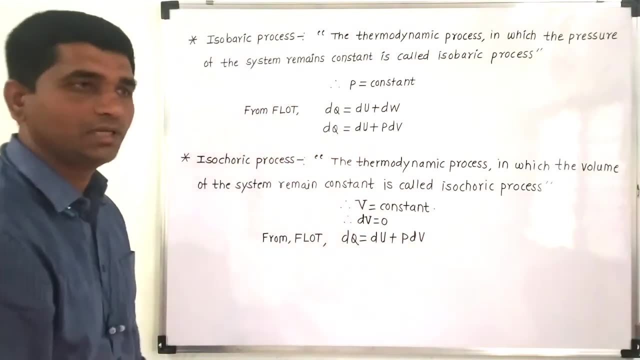 but, as in this case, for an isochoric process, what do we have? as volume is constant, so change in volume: it will be zero. so change in volume, it will be zero. so as change in volume, it will be zero. so in this case, dQ is equal to. 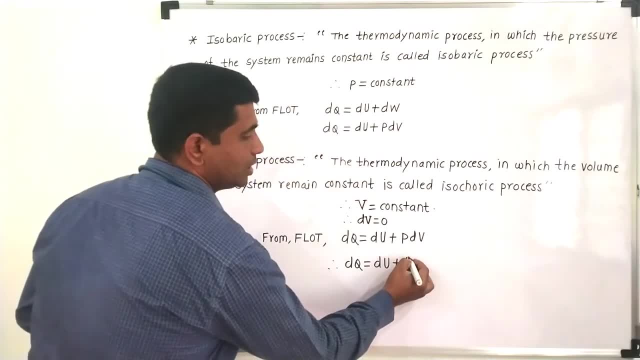 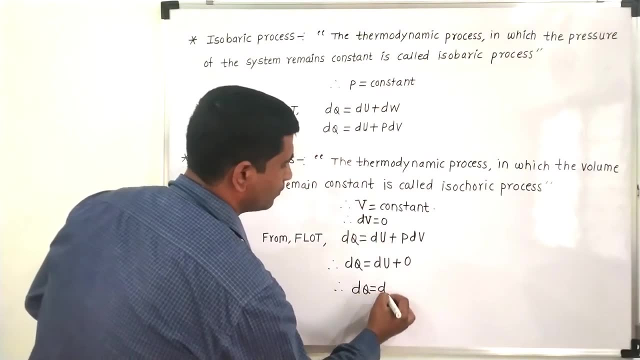 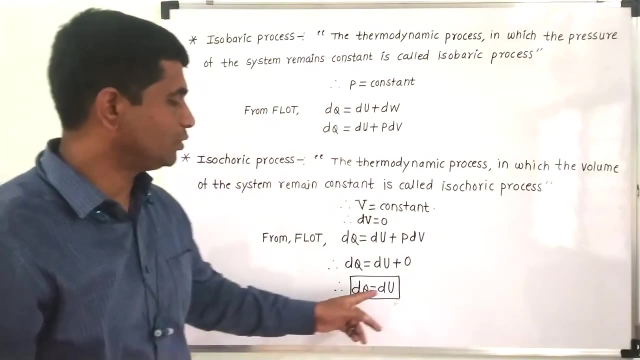 this will be dU plus zero, because dV it is coming out to be zero. so from this one we can rewrite that whatever the amount of heat it is given in case of isochoric process, it will be used only for to increase its internal energy. 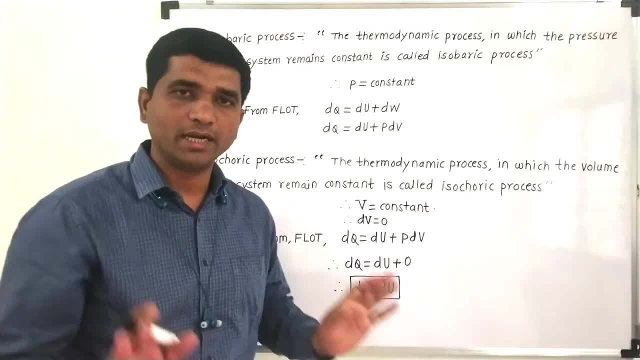 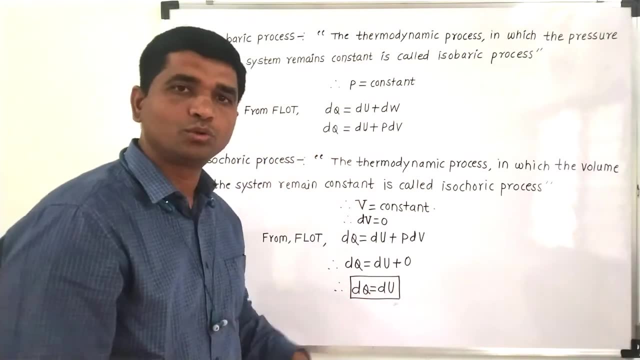 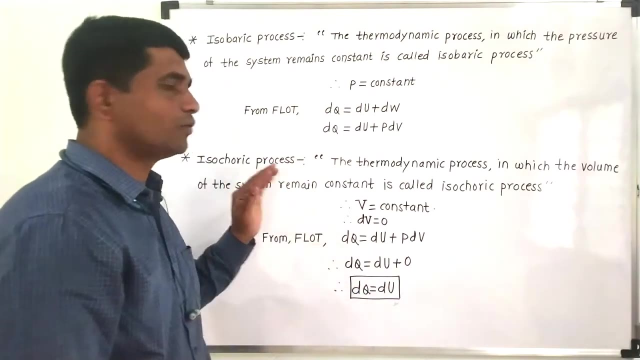 so in isochoric process we are not getting any kind of a bottle, we are just getting. whatever the amount of heat it is provided, it will be used to only increase its internal energy. so that is the significance of a first law of thermodynamics for an isochoric process. 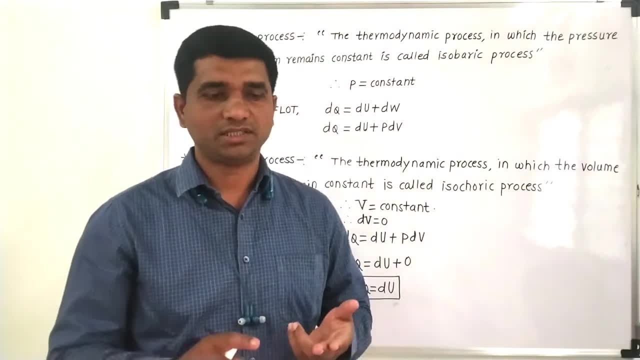 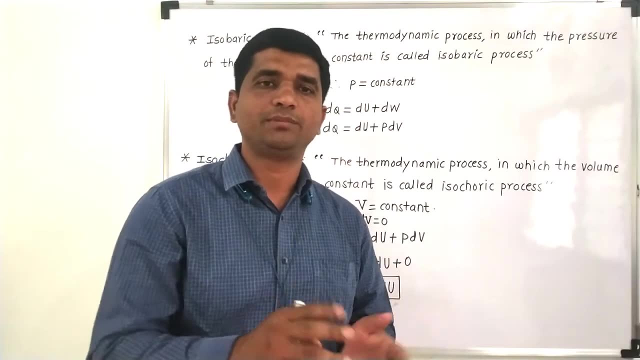 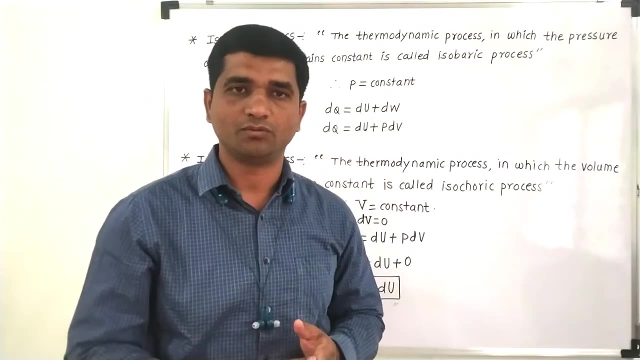 so, basically, in today's session, what we have discussed is: we have discussed what is first law of thermodynamics, which states that the amount of heat given to the system it is used for the two purposes. the first purpose is to increase its internal energy and second one is to perform some external work. 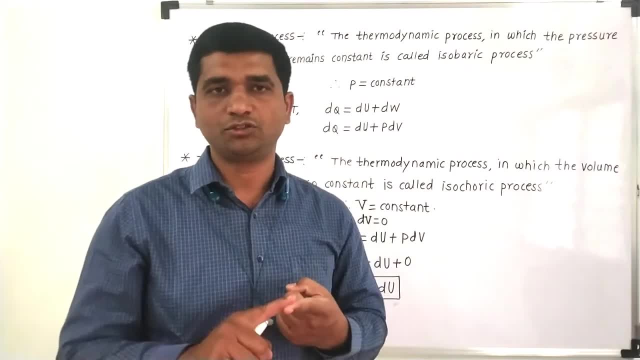 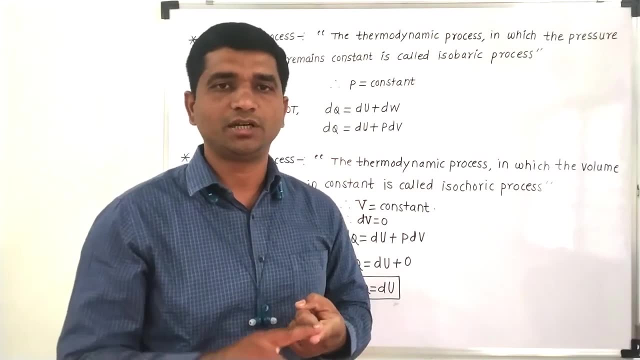 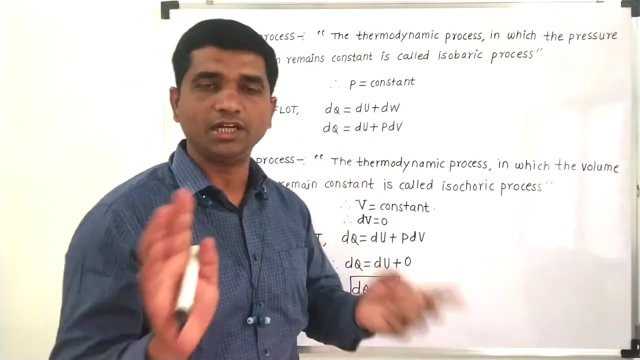 we have applied the first law of thermodynamics for the isothermal process. for isothermal process temperature remains constant. as temperature is constant, so change in internal energy will be zero. so whatever the dQ this first law of thermodynamics reduces to. dQ is equal to dW. 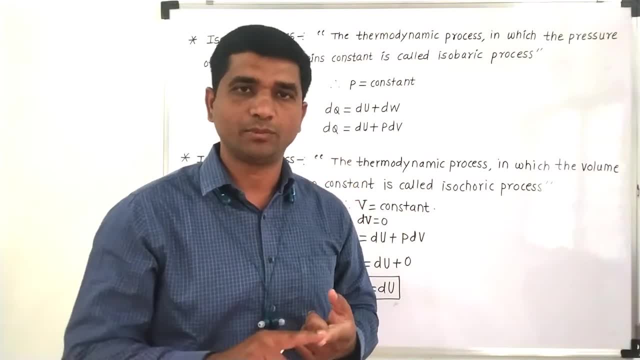 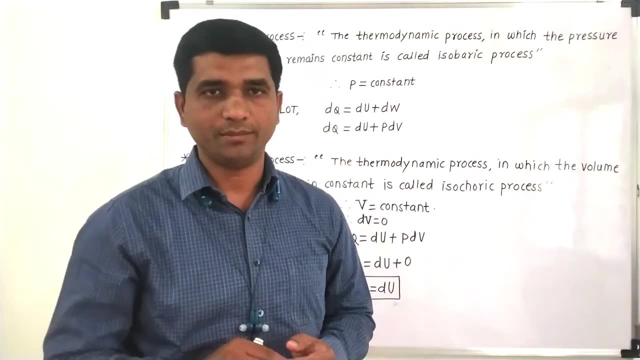 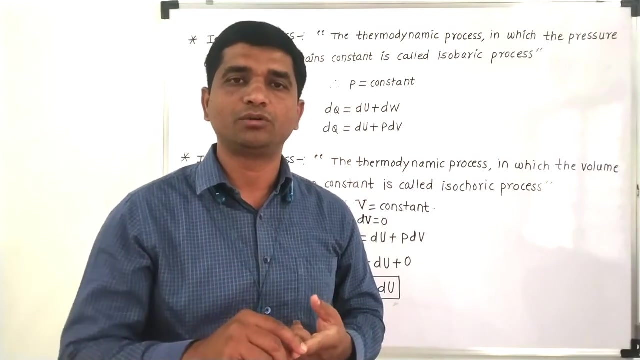 so means in isothermal process we are getting a maximum work done. this maximum work done in an isothermal process we will be calculating in our coming lecture. after that we had seen what is adiabatic process. in adiabatic process, the amount of heat given to the system.